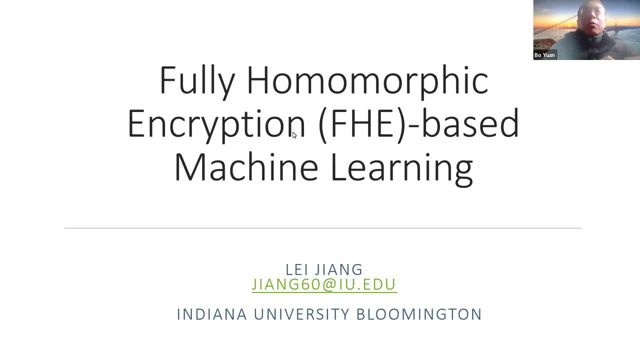 Hello everyone, so welcome to our this week's Progress in Future AI seminar talk and this is our first talk in the new semester. Today we're very glad to have Professor Lei Jiang from Indiana University, Bloomington, to give us this talk. Professor Jiang is currently Assistant Professor in the Department of Intelligent Systems Engineering at Indiana University. 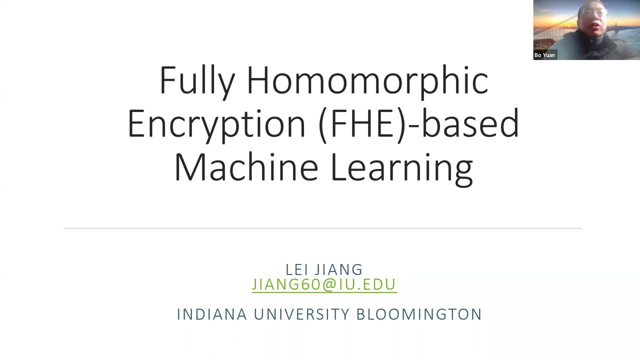 He obtained his PhD from the University of Pittsburgh and a Bachelor degree from the Shanghai Jiao Tong University, And his research interests include the hardware accelerator design and the privacy preserving machine learning, And he has done a lot of the very pioneering work in this- the privacy preserving machine learning and algorithm and hardware co-design- and published many wonderful works in the neuropsychology and so on. 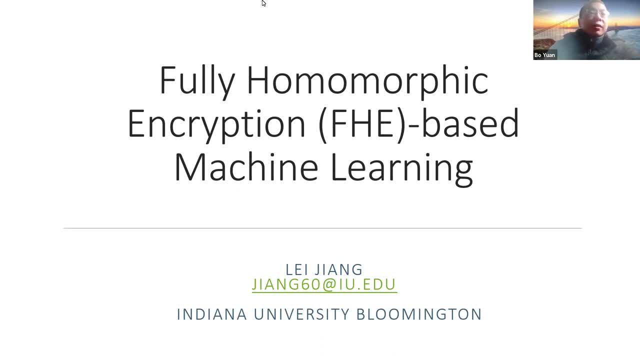 So now let's welcome Professor Jiang to give us this talk. Okay, thank you very much for your introduction. Thank everyone here for attending my presentation. I'm very glad to share our work on fully homomorphic encryption-based, FHE-based machine learning today here. 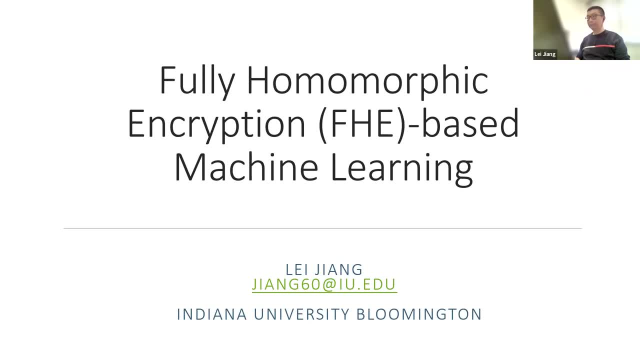 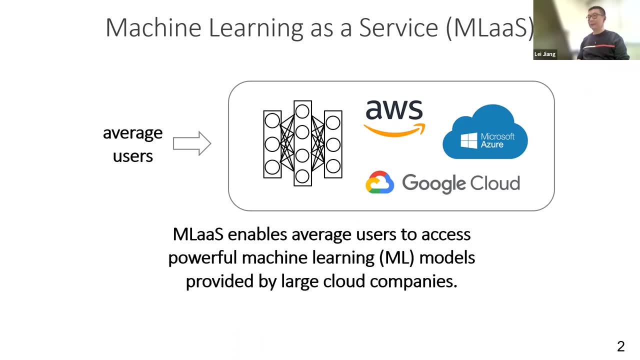 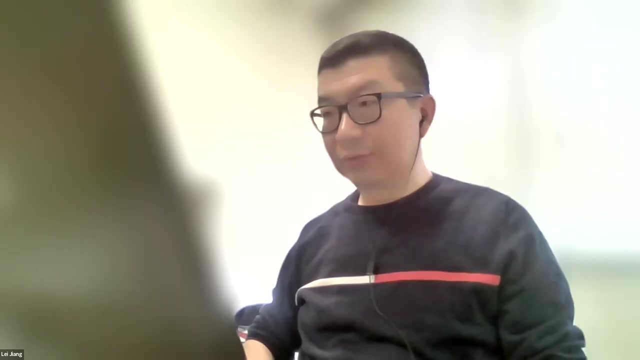 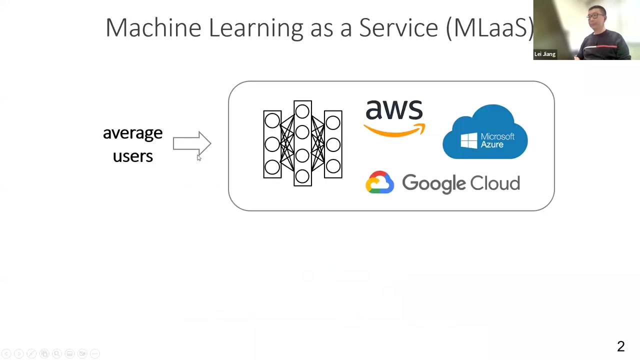 So let's start. I think nowadays, the machine learning. machine learning is the dominant approach to solving a wide range of problems, such as computer vision and natural- I'm sorry, natural- language processing. I need to re- reset this. I need to re-reset this. 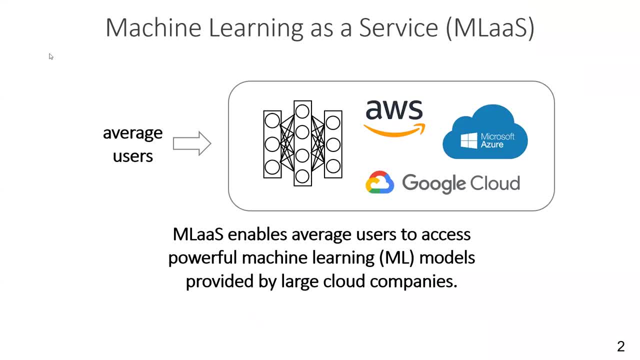 Now, So I can see your screen. Yeah, Okay, nowadays the machine learning is the dominant approach to to solve a wide range of problems like computer vision and the recommender system. However, it's very difficult for the average user. 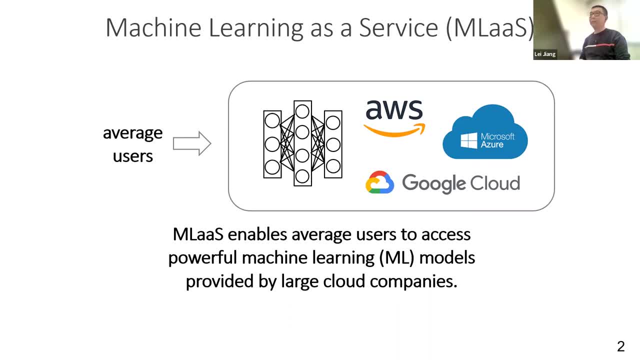 to train a neural network themselves. This is because training a powerful and accurate motion learning model require, first, a lot of training data. Nowadays the training data can be at a terabytes level. Second, super long GPU hours If you want to train a transformer. 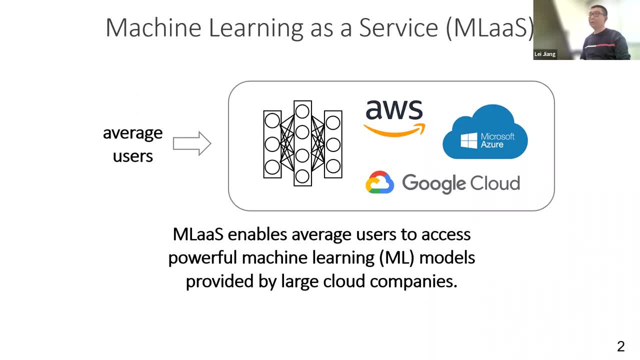 then basically you need tens of GPU to run maybe four weeks. Last but not the least, you also need a rich domain expertise. What type of regulation method you need during the training is a big problem. So that's the reason why average user cannot train. 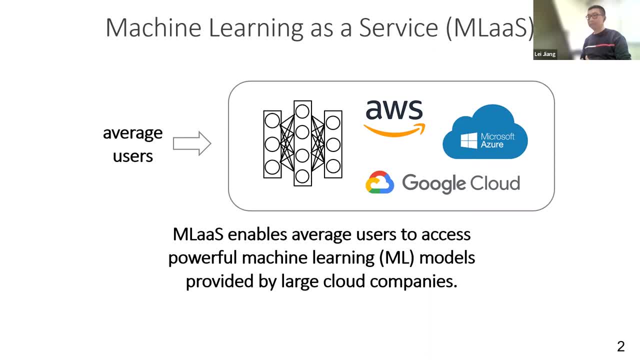 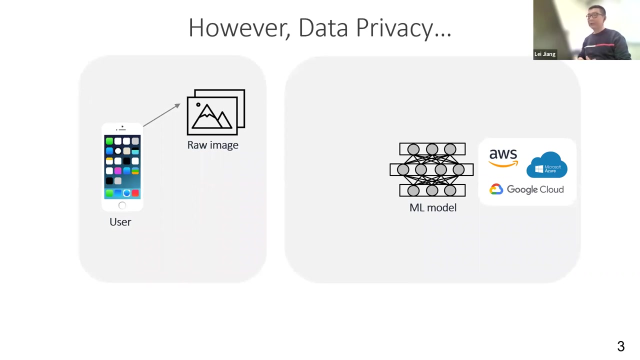 an accurate and powerful model themselves. Motion learning as a service is a very effective method to enable average user to access the powerful and accurate neural network model in the cloud produced by large cloud computing companies like Google, Facebook and Microsoft and Amazon In the process of machine learning as a service. 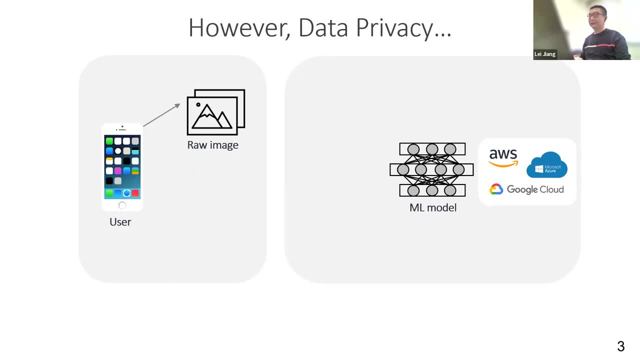 the user can just send his or her raw data, input data, to the cloud And then the server can do the inference directly on the input data and the generator and output and send the output back to the user. So during this process actually, 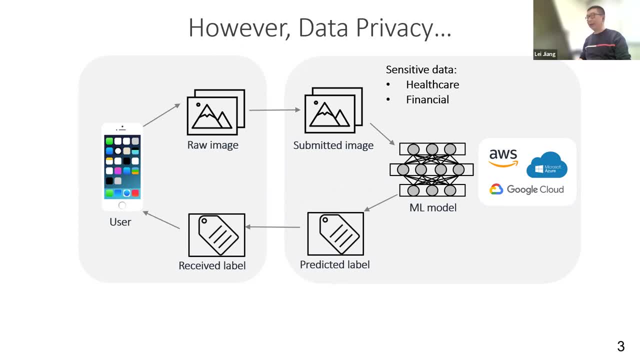 the server can be very Ip. industrially server can know the input and the output. so it's a very relevant for average user to share their private data like a healthcare record or any financial data. no, nobody want to do that nowadays. the government regulation even forbids the private data sharing between clients. 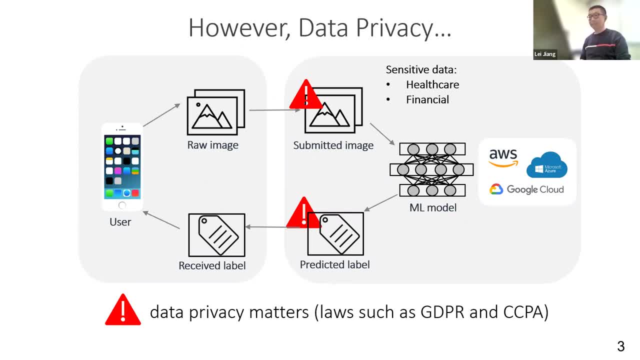 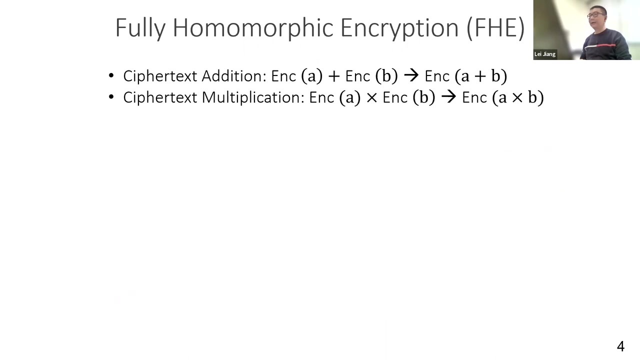 and some large companies like the ccpa and the california consumer privacy act and some european laws. so it's really important to make sure we have very good data privacy in the machine learning as a service without a fully homomorphic encryption. fhe can help us to solve this problem most fhe scheme. 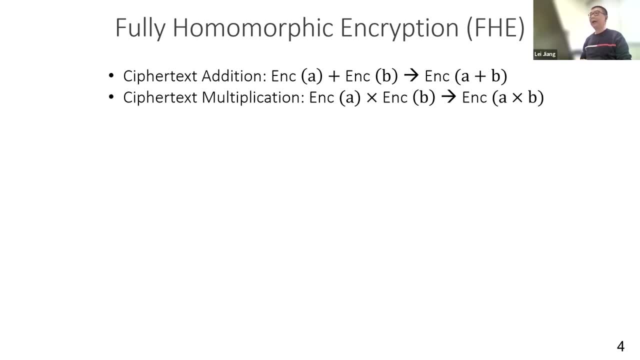 uh support cipher test addition and cipher test multiplication. so the idea here is very simple. the sum of two encrypted variables is equal to the encrypted sum of these two variables. we have the same thing for the multiply- multiplication. so during the cloud computing a user can do an addition on a and b locally. he or she can also encrypt the a and encrypt the b and. 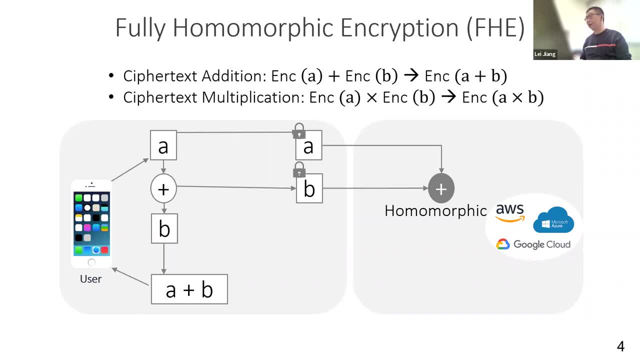 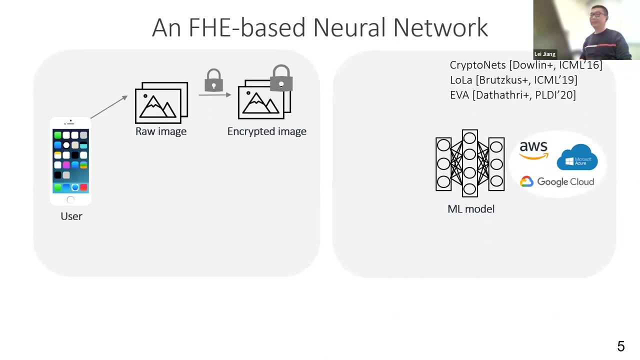 send only two cipher tests to the server in the cloud and the server can do an addition homomorphically and then return the encrypted a and b. so these two values should be the same. beyond simple addition and multiplication, prior work also create an fhe based neural network. 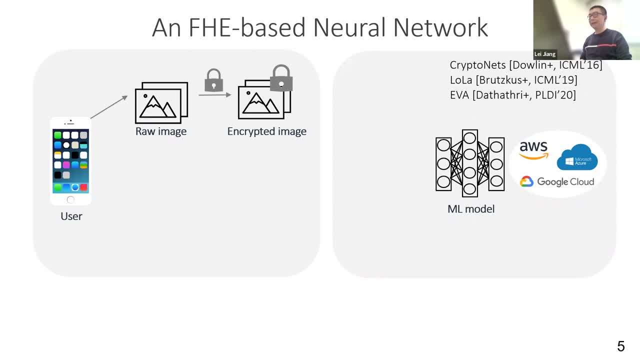 for machine learning as a service. so the in the context of machine learning as a service, a user can encrypt his or her raw input into c szer tests and send only the c bereits to the server in the cloud and then remember that theques test two ipad test that can be used to functionally in a machine learning as a service. so in the context of machine learning as a service, a user can encrypt his or her raw input into cipher tests and send only the c ном Grams, only the c four tests to the server in the cloud And then the SQL components report the table. 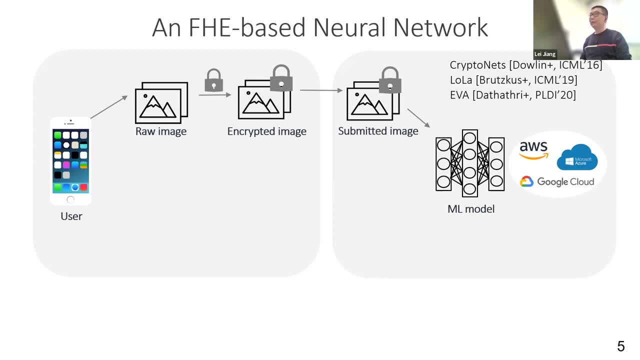 dear patients, thank you very much. see, Beth, thank you for watching. server can do computation homomorphically on the cipher test and generate an encrypted output and return this output back to the user. Only the user has the secret key, so only the user can do the decryption and know the results. 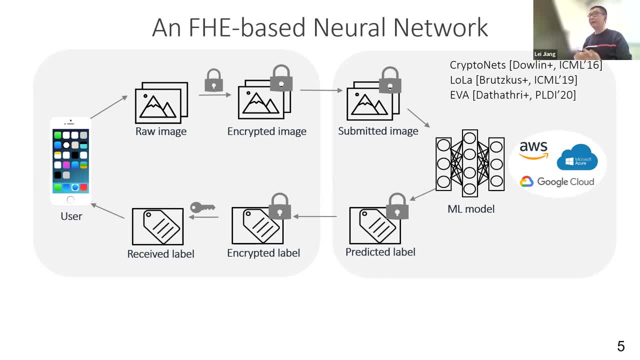 So during this process we have an end-to-end FHE encrypted data flow. So this encrypted data flow can protect the data privacy of the average user During this process of machine learning. as a service with FHE-based neural network, it's very flexible for the user. 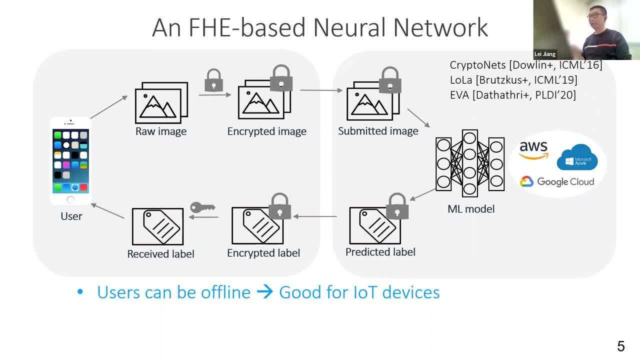 The user. the user can even go offline during the computation, after sending the cipher tests to the server, because there is no frequent communication between the server and the user during this process. So it's very good for the IoT devices. Again, we don't have too frequent communication. However, the FHE is very time-consuming. 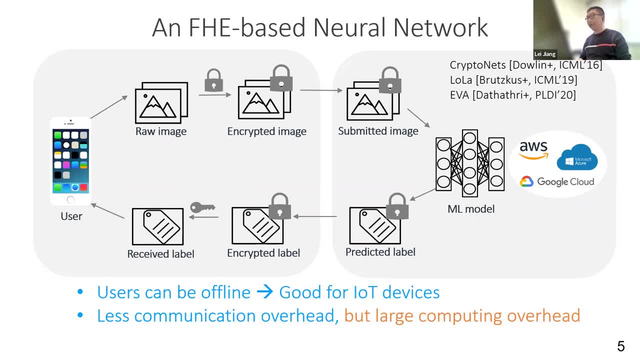 And very complex, computationally expensive, So we need to spend a lot of time in computing the FHE-based scheme. Another disadvantage of FHE is that it cannot support the non-linear operation well, which means that if we use FHE to 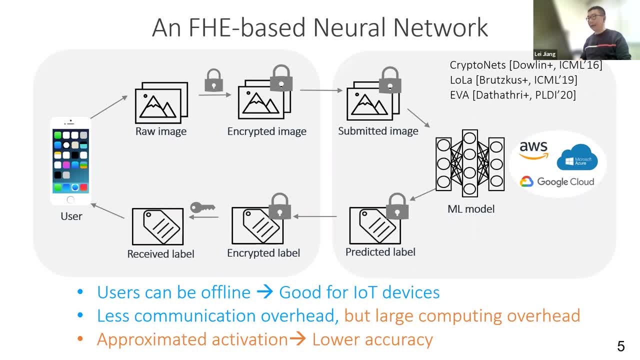 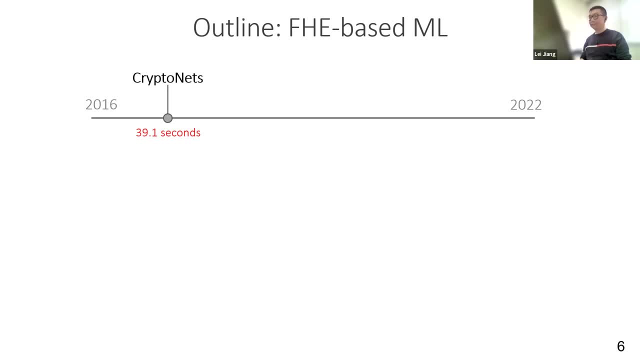 implement a neural network. the accuracy may not be high, So the first FHE-based neural network is called CryptoNets, which is created by Microsoft. It spans 40 seconds to inference an MNIST image, a very small image actually. 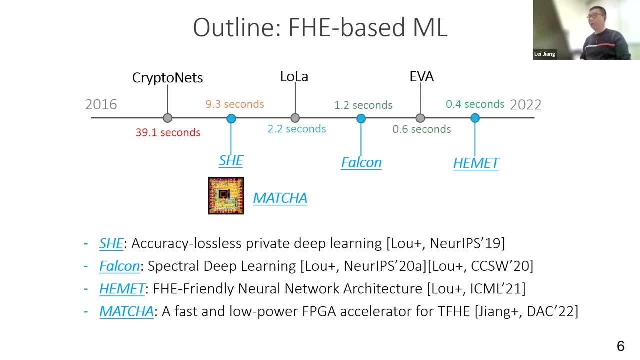 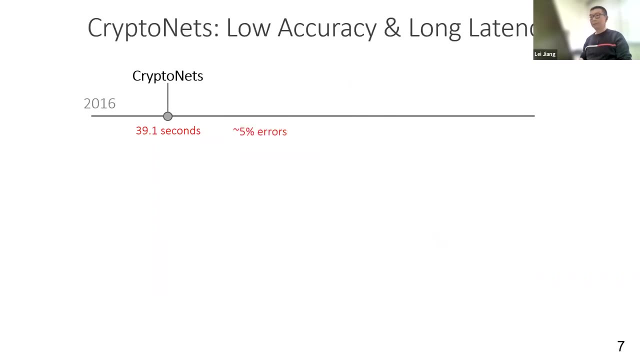 So in this talk I will introduce four works, recent works from my group. Three of them are algorithm work. The last one is hardware-level work. So one inference- FHE-based inference- of CryptoNets on a small MNIST image cost nearly 40 seconds. 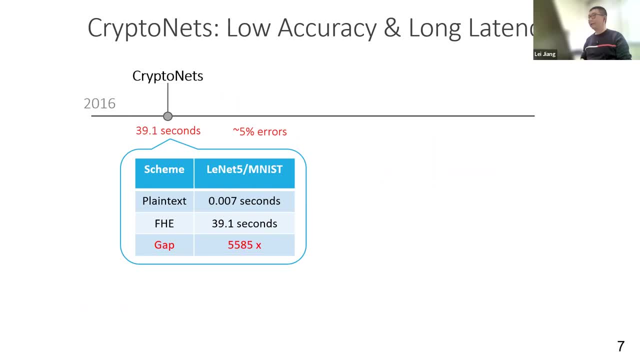 However, if we do the same thing on the plan- test unencrypted data- it costs only less than 0.01 second. So there is a more than 5000 times latency gap Beyond the latency long latency, the accuracy of the FHE-based neural network is not high either. 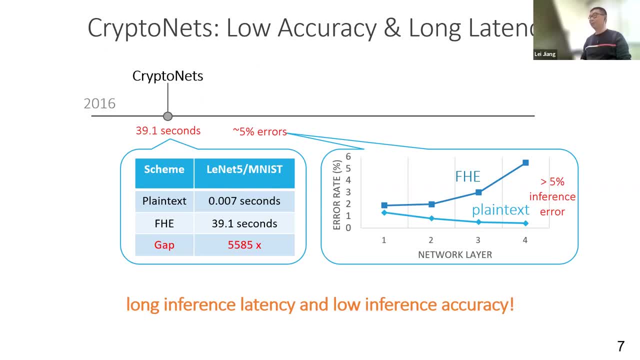 For a plan test: neural network for unencrypted data. if we try to integrate more and more layers into the neural network, the accuracy should go up and the error rate should go down. This is so-called deep architecture- deep neural network architecture. 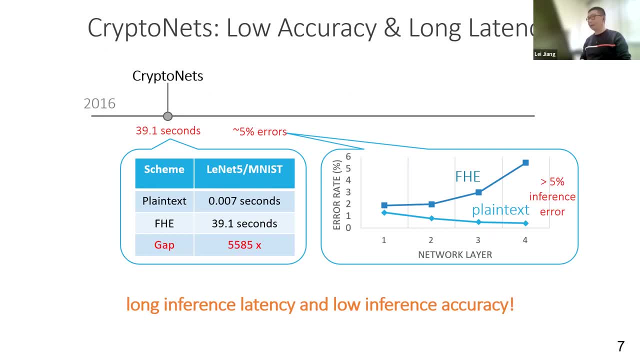 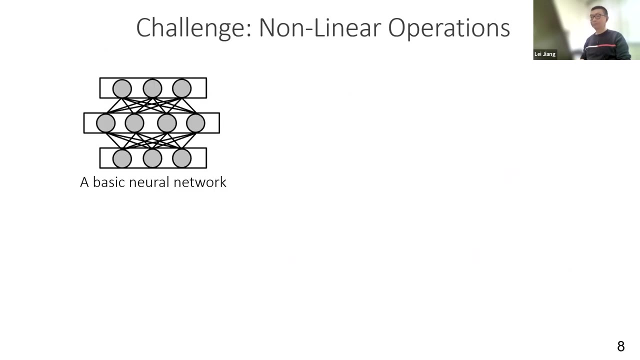 However, if we do the same thing for the FHE, then the error rate actually goes up. I will explain why we have this phenomenon. So we need a low latency and a high accurate, high accuracy neural network. And here is one very simple example of a neural network. 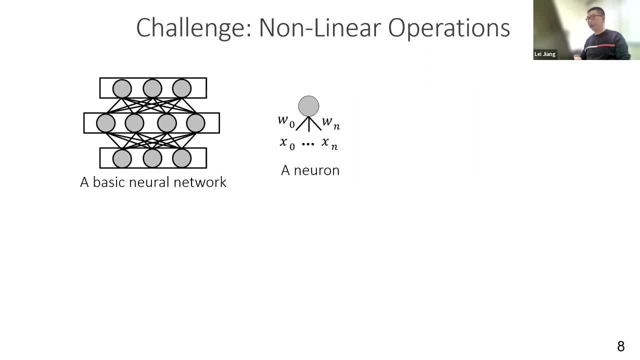 The fundamental unit is actually a neuron. In a neuron we have multiple weights and we also have multiple inputs. So during the inference we need to compute the multiplication between inputs and weights. We need to compute the multiplication between inputs and weights. 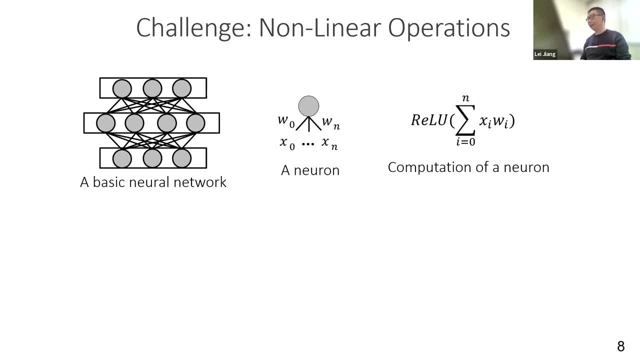 And the result is the number of elements of the neural network, And we need to compute the multiplication between inputs and weights. To do this we need to write a formula. We will compute the result and then sum all the intermediate results together. 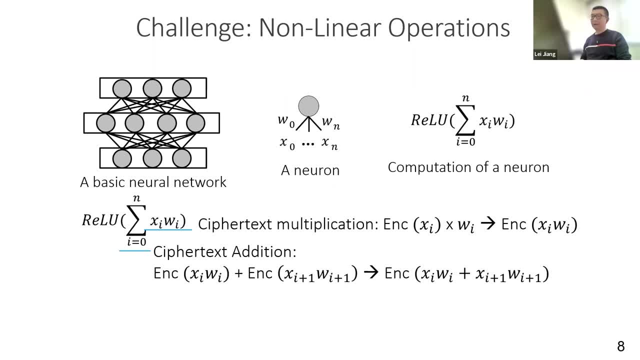 and then do a nonlinear relu activation on the final result. So the FHE for most FHE schemes they have no problem with the multiplification and accumulation because they can support a multiplication and addition on the CIFER test. However, for the nonlinear relu, 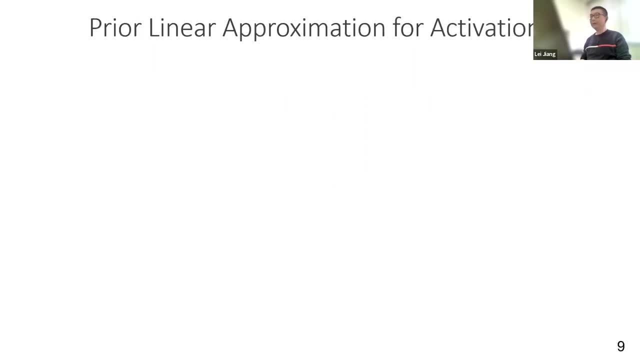 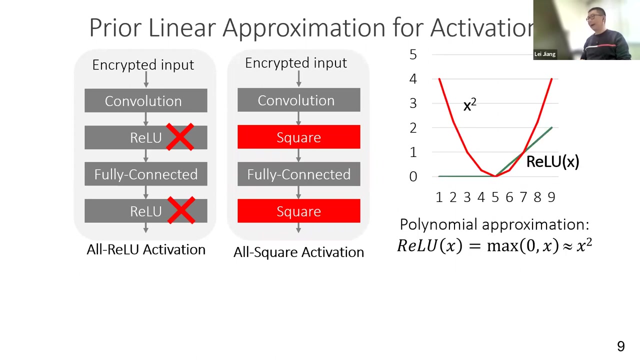 scheme has difficulties. so this is the reason why crypto nets actually replace all the relo in a neural network by square function. the square function is x to 2, which is actually a degree two polynomial. they actually use this degree two polynomial to approximate the relo operation. 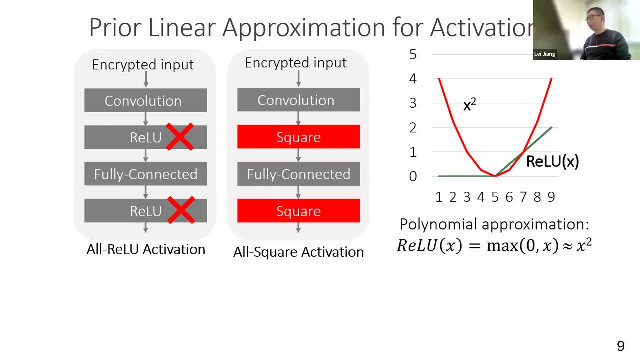 although the square function can bring some non-linearity, you can see there is a huge difference between these two curves and that's the reason we will have a lot of error in the activation layer. so if we stack multiple activation layer together, the error will be enlarged. 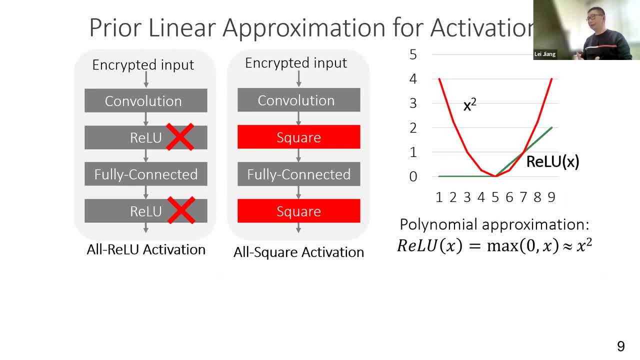 that's the reason why when we try to integrate more and more layers and the fhe based on your network actually has lower accuracy. so when you see the degree two approximation polynomial here one very simple question- you may ask how about to use a higher degree polynomial to approximate activation? 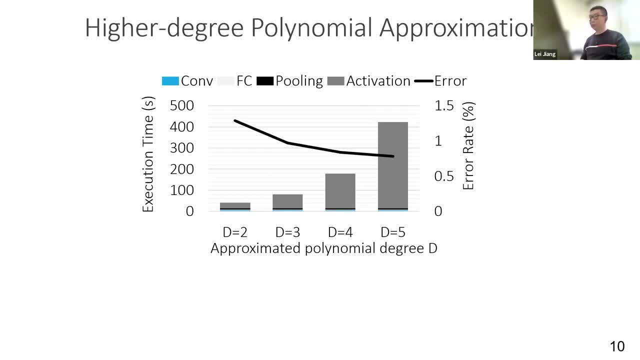 we try that we actually use the degree two, degree three, degree four and five approximation polynomial to approximate the activation. we can see that from this figure the error rate actually slightly decreases and so the higher degree approximation polynomial actually works. unfortunately, and the execution time of one inference. 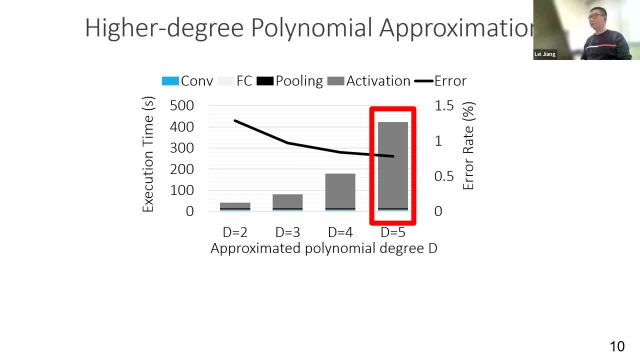 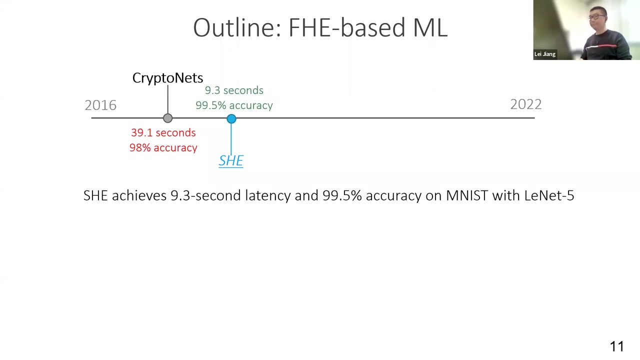 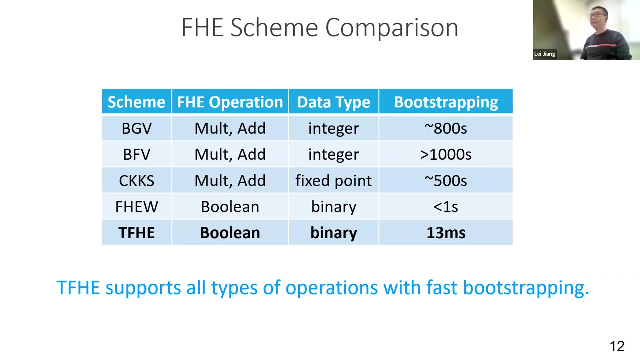 also significantly increases. now 99 percent of the latency is actually consumed by the degree five approximation polynomial activation. this is not good. we need a fast and accurate reloop. then we propose our first technique, she. so the fhe's principle can be implemented by many schemes, including some worldwide scheme like a bgb. 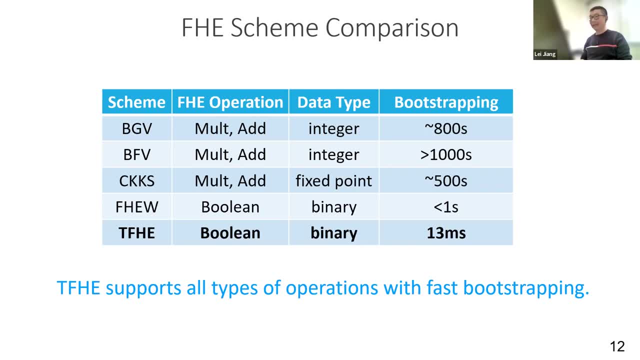 bfb, ckks. they support a multiplication and addition. we also have some so-called bitwise, fully homomorphic encryption scheme like tfhe and hew, because the tfhe is faster. so in this talk i mainly focus on the tfhe, so the tfhe can support a homomorphic boolean algebra. 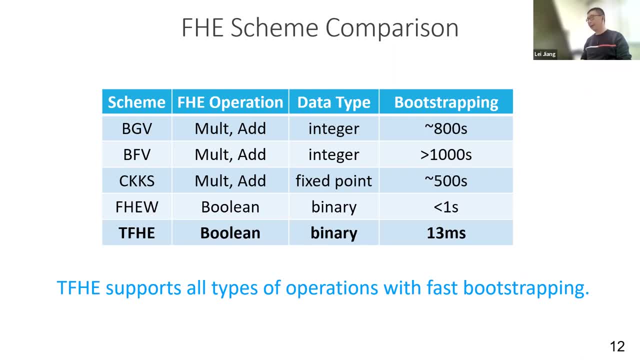 like a homomorphic xor gate or homomorphic non-gate. by these binary logic gates we can build any computation we like by tfhe gates. so tfhe is more powerful than the worldwide fhe scheme like bgb, bfb, ckkf for those worldwide fhe schemes. 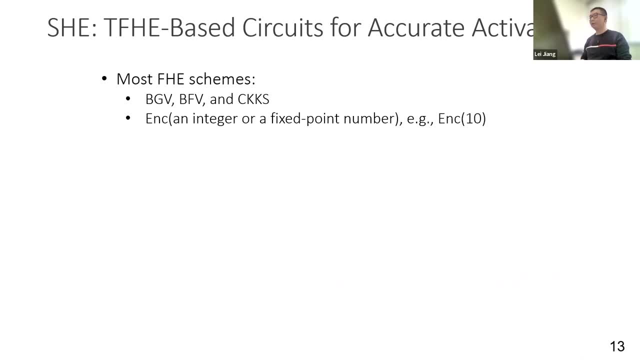 scheme, they encrypt an integer or a fixed point number as a whole. So if we have an integer 10, then they can encrypt this 10 as one number. However, if we use TF-HE to process this integer, we need to decouple this integer into four bits, and TF-HE only supports one bit. 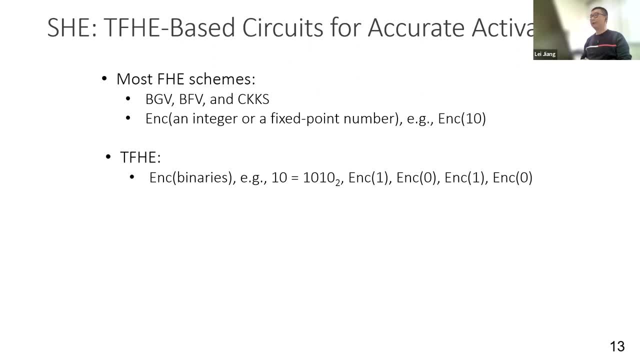 message. We need to encrypt each bit independently. So here we have a full CIFAR test actually, And then we can perform homomorphic logical operation on the CIFAR tests. By homomorphic logic gates. we can easily build a circuit to compute the ReLU operation. 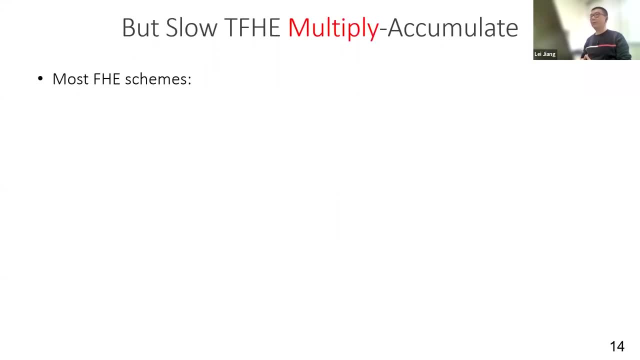 So if the TF-HE is so good, why PyroWorks didn't use it? The answer is no. If the TF-HE is so good, why PyroWorks didn't use it? The answer is no: If the TF-HE is so good, why PyroWorks didn't use it? 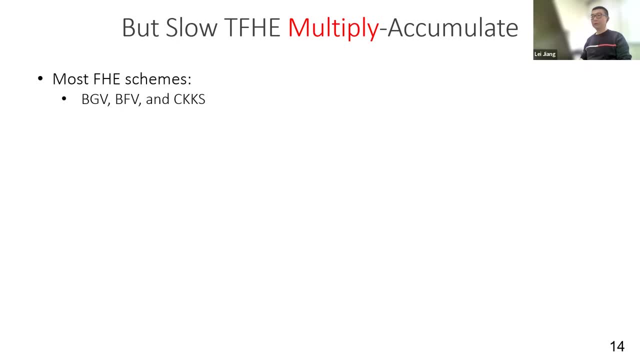 If the TF-HE is so good, why PyroWorks didn't use it? The answer is very simple. So for most worldwide FHE schemes, one multiplification can be done by one homomorphic multiplification. It's just one operation. 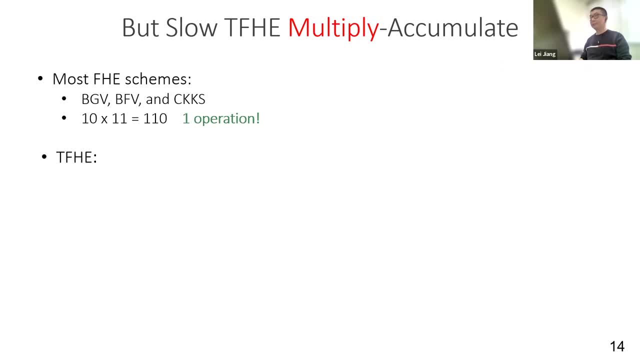 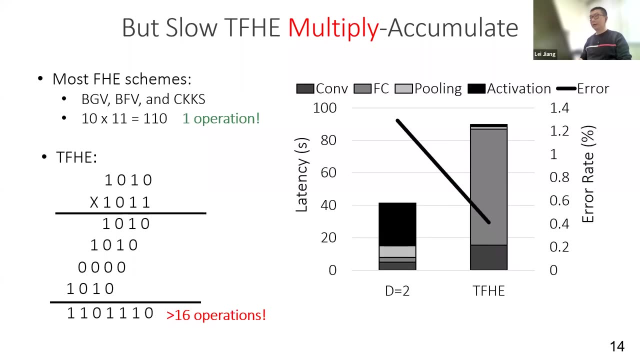 However, if we use TF-HE to compute the multiplification, we need to break this operation into more than 16 operations, So the multiplication on TF-HE is actually very slow. If we naively use TF-HE to build a neural network, although, the error rate will be very low, 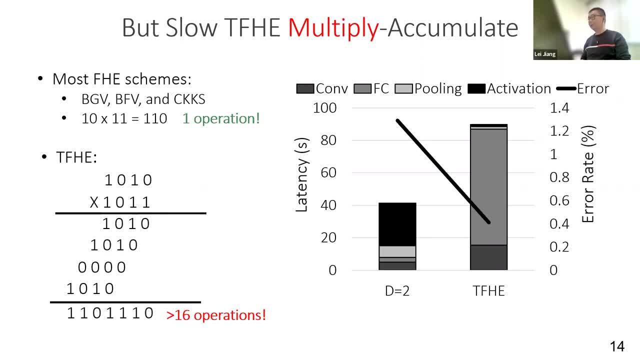 and the latency of the inference also will be significantly increased. From this figure we can see that actually the bottleneck of the TF-HE-based neural network is from the convolution layer and the fully connect layer. These two types of layers has a lot of multiplifications. 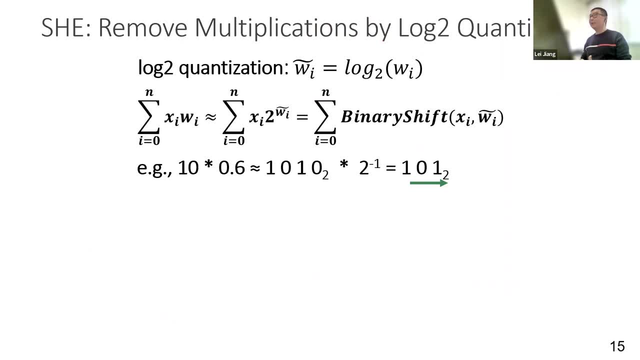 So one simple idea is that it can be reduced or removed, the multiplication in the inference of a neural network. So we try to use log2 quantization to remove the multiplifications. We quantize each weight to its 2 to w representations. 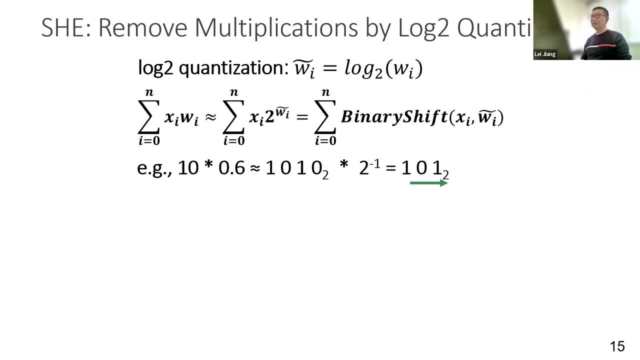 For example, if one weight is 0.6, then we try to approximate it into 0.5, which is 2 to minus 1.. A input 10 multiplied as 0.6 number is approximately equivalent to this 10 multiplied. 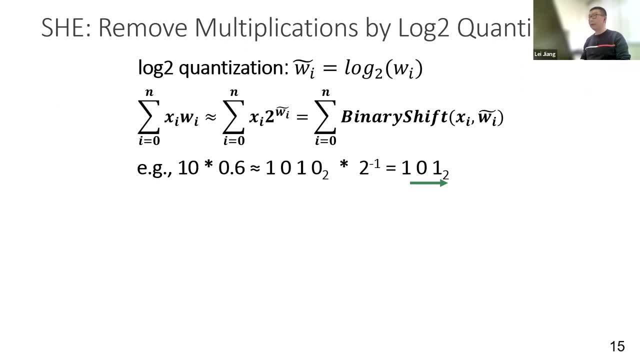 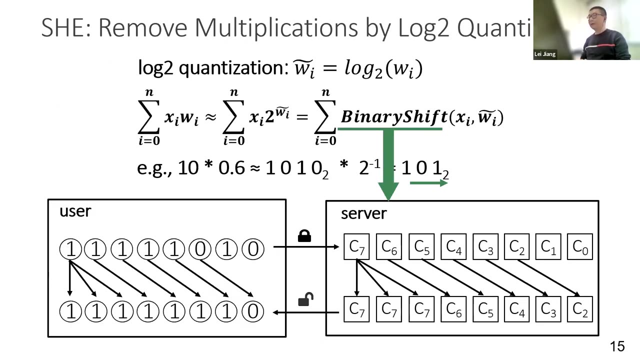 0.5, which is 2 to minus 1.. Then we can do a right binary shift. We actually shift this number by the input to the left- I'm sorry, to the right by one bit, Because the TF-HE actually encrypts each bit independently. 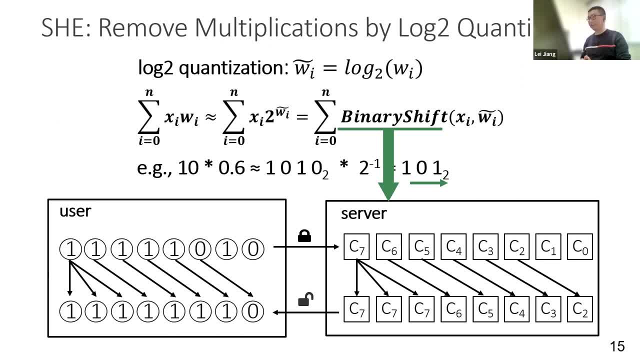 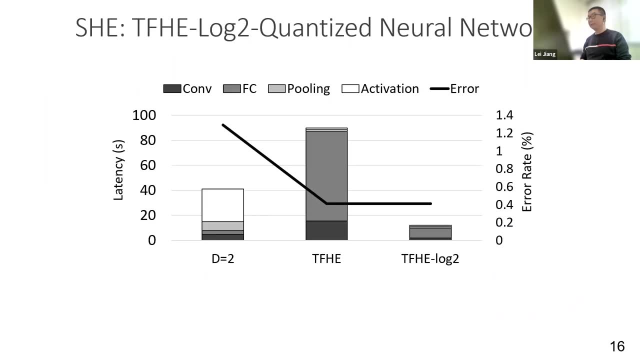 so it's very convenient for us to do the shift operation without very large overhead. Now the multiplication and accumulation will be converted to shift operation and accumulation. So in this way, when we apply the log2 composition and the TF-HE on a neural network, 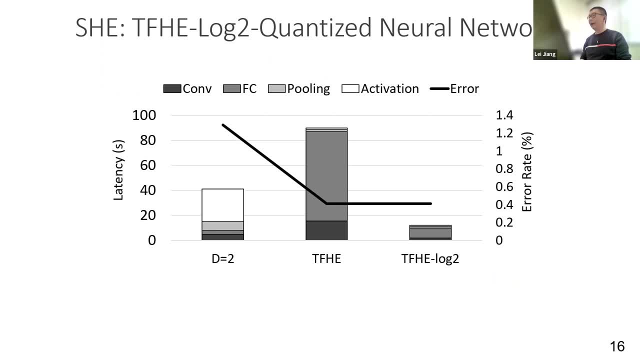 we can achieve very low latency but maintain the same accuracy as the TF-HE neural network. So now we can reduce the inference latency of an MNIST image to 9.3 seconds. So the TF-HE is now able to do the shift operation. 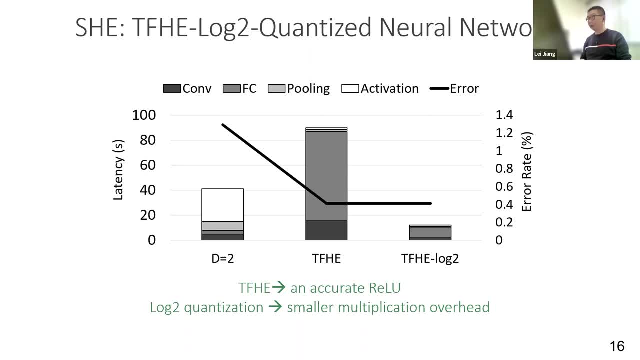 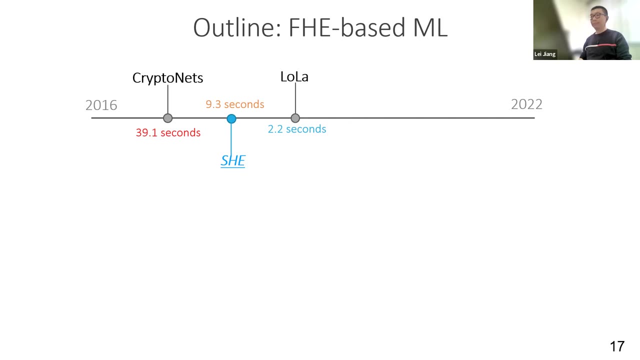 and the TF-HE can help us to achieve a very accurate relu operation, And the log2 composition can help us to reduce the overhead of multiplications. By these two techniques, we can reduce the inference latency on an MNIST image to 9.3 seconds. 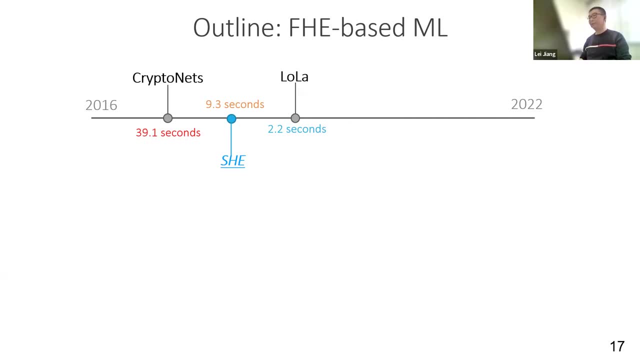 Our work also proposes another approach based on a FHE-based neural network called LALA. It can reduce the latency of this MNIST image to 2.2 seconds. Now the gap is approximately more than 300 times LALA actually takes advantage of the batching operation. 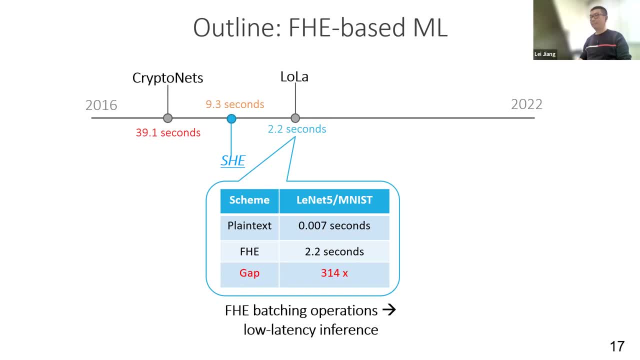 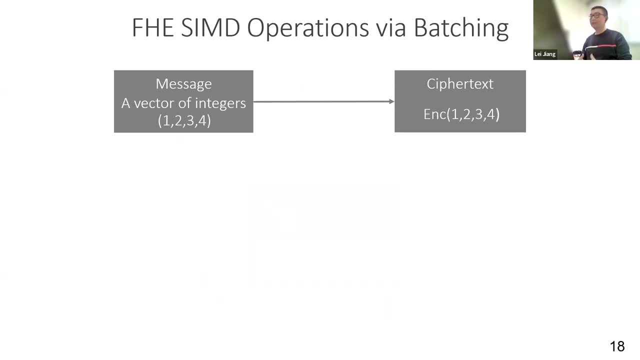 to achieve low latency by FHE-based scheme. So when you have multiple integers for the worldwide FHE-based scheme, you can actually encrypt these numbers into one single cipher test And then we can perform so-called single instruction, multiple data computation on the cipher test. 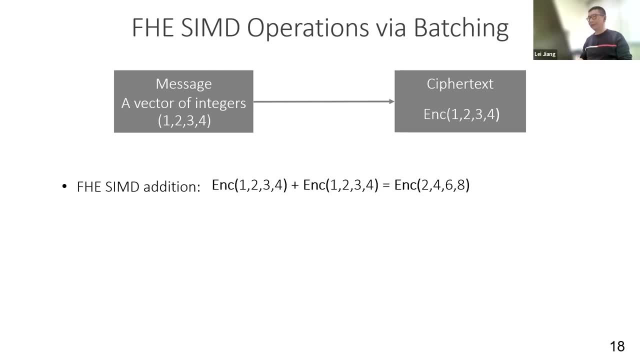 So when we perform a homomorphic addition on two cipher tests, between two cipher tests, we actually perform four, three additional additions on each number slot. In this particular example, we have one plus one, two plus two, three plus three and four plus four. 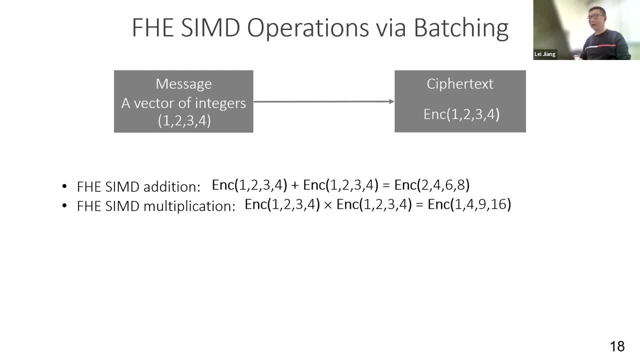 We have the same thing on the multiplication part. This is good because we actually batch multiple integers into one single cipher test. We also need a rotation operation And the rotation operation. the rotation can actually move the number slot inside a cipher test by some offset. 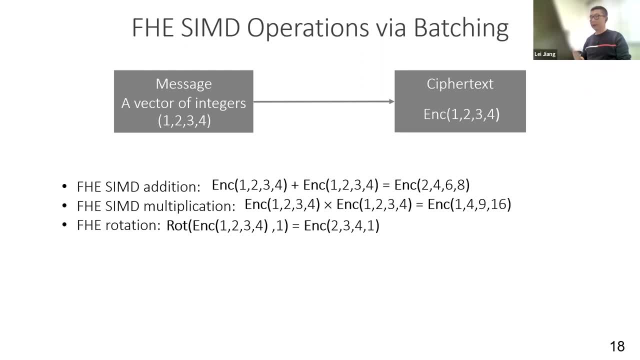 In this example we just move all the number slot to the left by one slot, Now the two. that number two is the first element in the cipher test, But the number one is the last number in the cipher test, So the so-called SIM. 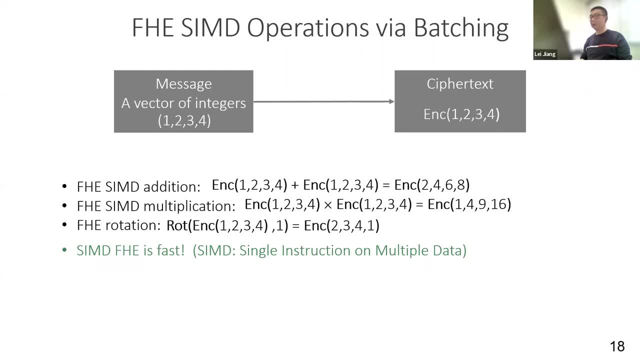 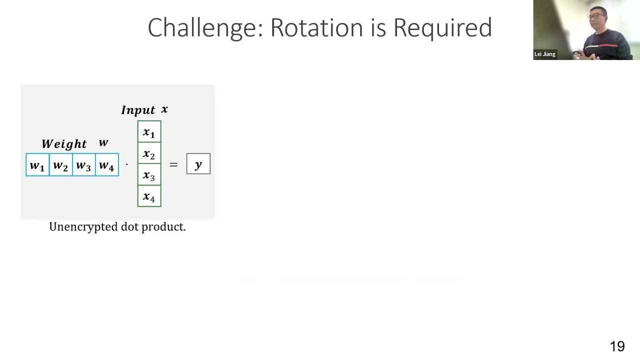 the computing style is very good. Potentially we can achieve thousands of throughput improvement, But the rotation is very slow. particularly the matrix vector multiplication need a lot of rotations. So this is what we typically do for the plan test vector matrix multiplication. 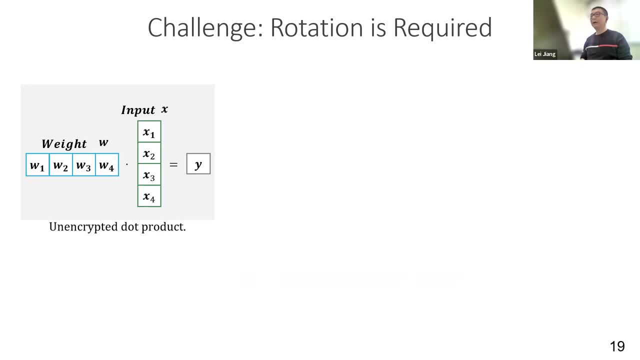 So this is what we typically do for the plan test vector matrix multiplication. We just do the multiplication between W and X and then accumulate the results together. However, if we want to do this in the FHE domain, we need to encrypt the W into a cipher test. 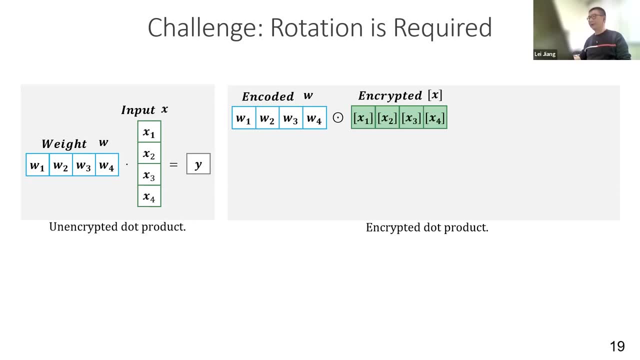 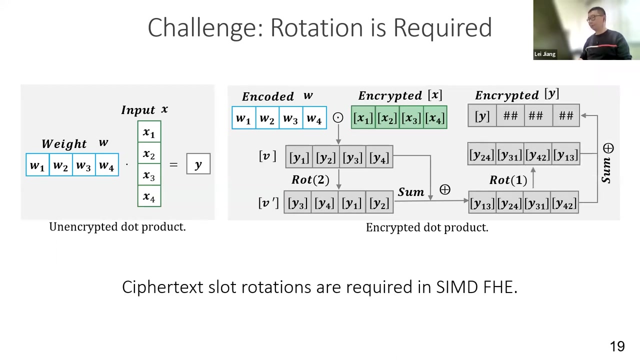 and then the X into another cipher test and then do a SIM, the multiplication between them. After we have the intermediate results, we needed to do the rotation and then do SIM and then continue to do the rotation and the SIM until we have the final output. 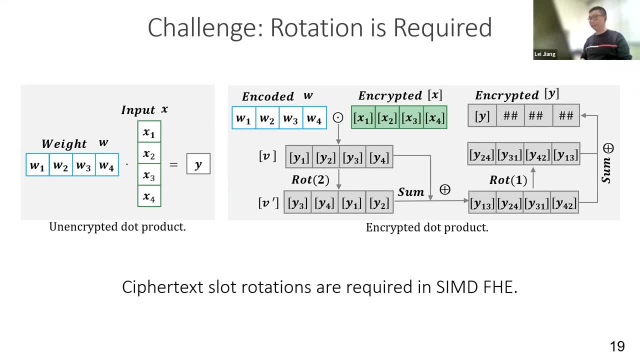 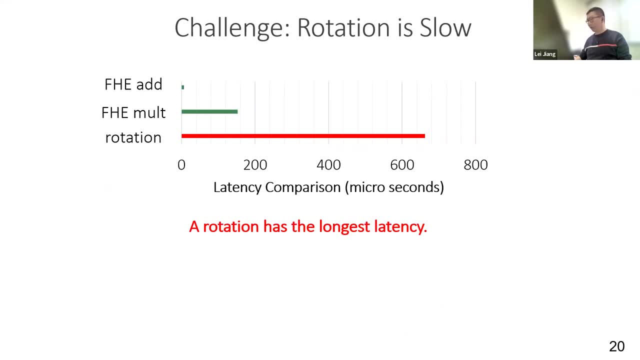 So during this process we need a lot of rotations. Unfortunately, the latency of the rotation is very long. It's much longer than the FHE. Unfortunately, the latency of the rotation is very long. It's much longer than the FHE. 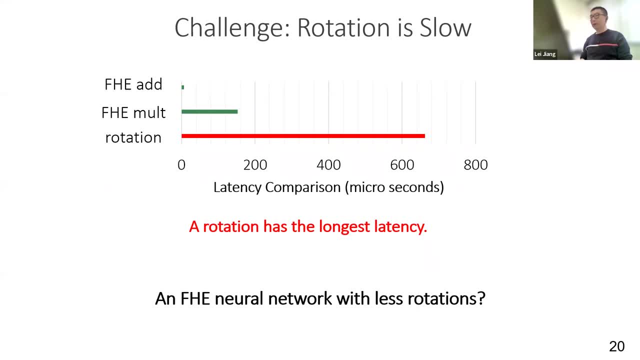 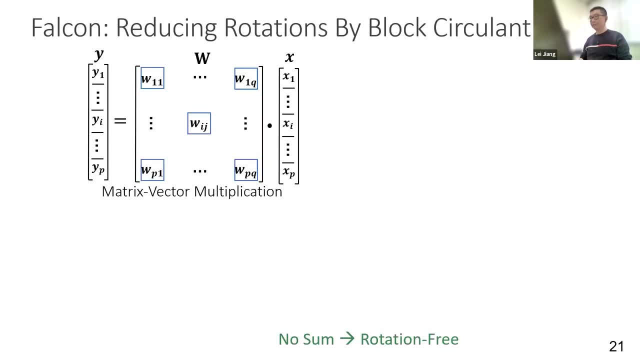 So we need to do the multiplication. So we need to do the multiplication. So one natural question is that: can we reduce the rotation in a neural network? The answer is yes. We can continue to use the composition to count as the weights. This time we can count as the weights. 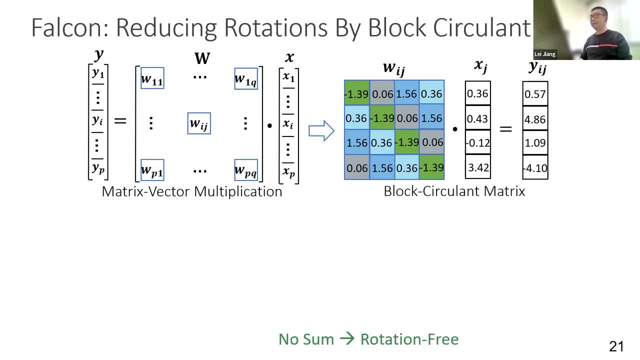 into a block circulant matrix. In a block circulant matrix, the matrix, we can use only one row to represent the entire weight matrix. for example, we have the first row and then we can do shift operation to generate the other rows. so during the vector, 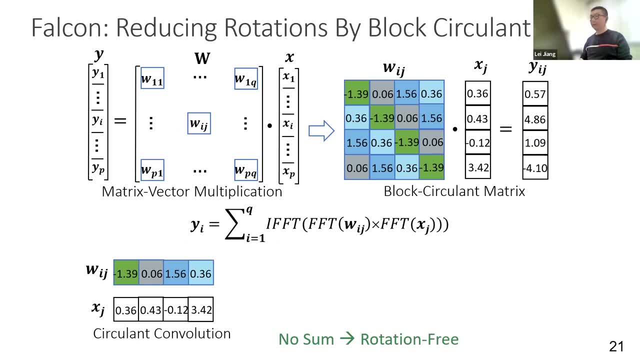 multiplication. we can do fft and inverse fft. we can perform fft on both the weight and the input and then do only coefficient, wise multiplications, and then a inverse fft can help us to achieve the final result, because in this example we do not have some operation, so we do not need rotation. 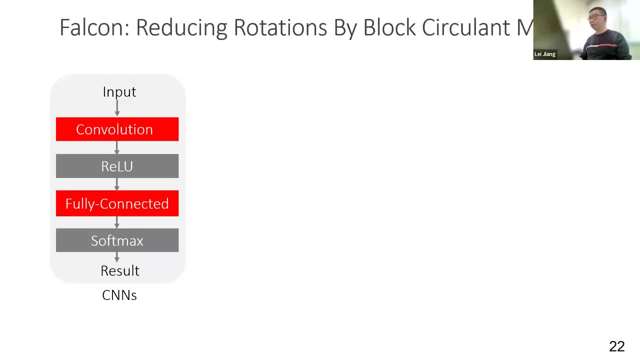 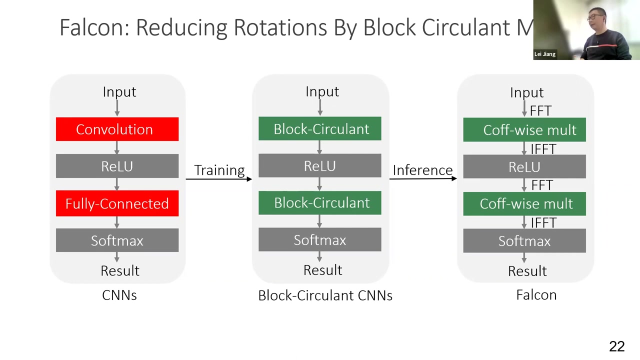 so during the training of a neural network we can countize the weights into different block circulant circuits, and this is this is we will do for convolutional layer and the fully connect layer. and then during the inference, we only do a small number of fft and inverse fft. 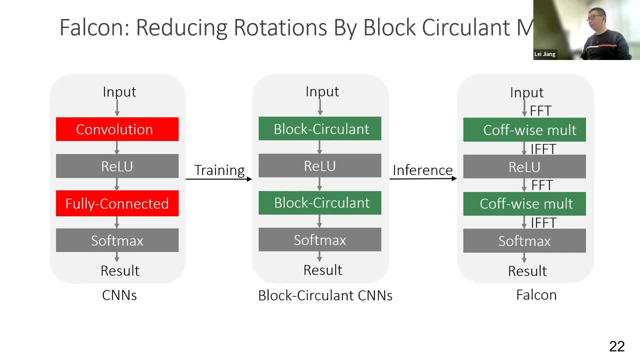 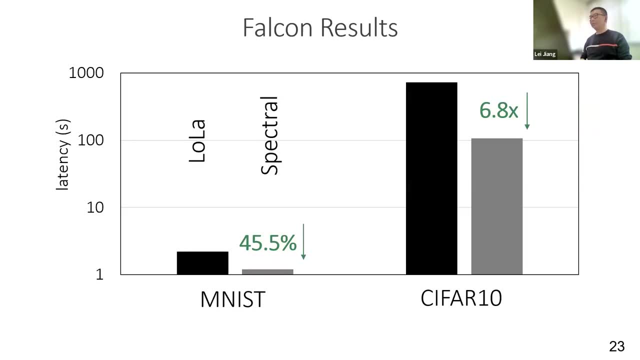 and then we can all do the coefficient wise multiplication without a large number of rotations. so by doing this simple block circulant based composition, we can reduce the latency of a amnesty image by 47. now the latency on a very small image is very short. then we can try some larger data set like c410. 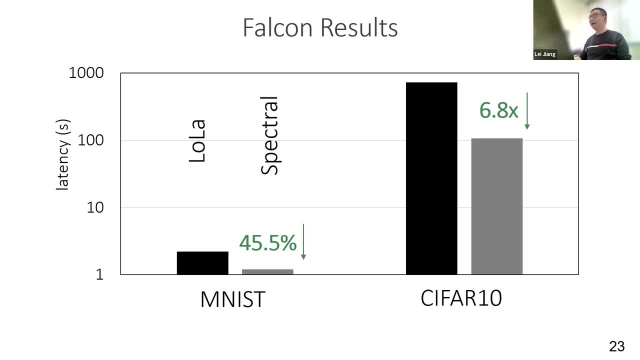 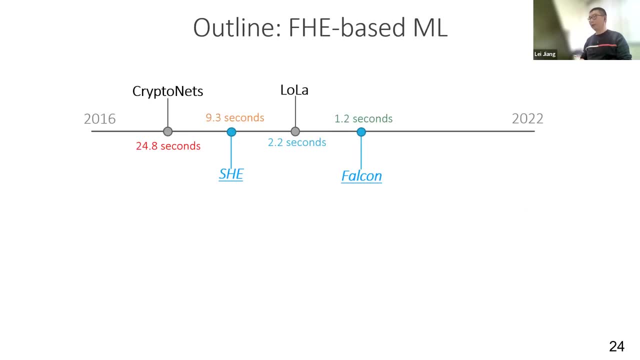 for a c410 image, we can reduce the latency by more than six times. so now our scheme can reduce the latency of a amnesty image to 1.2 second. a more recent prior work proposed eva to reduce this latency to 0.6 seconds. 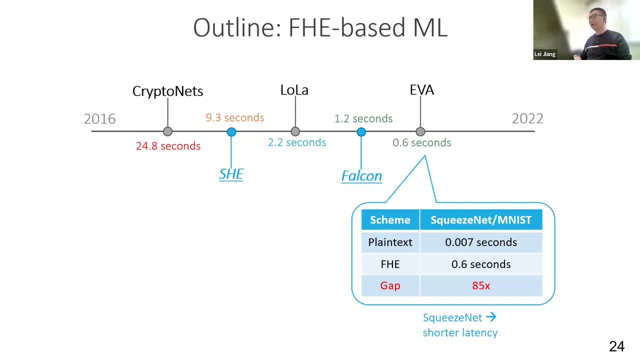 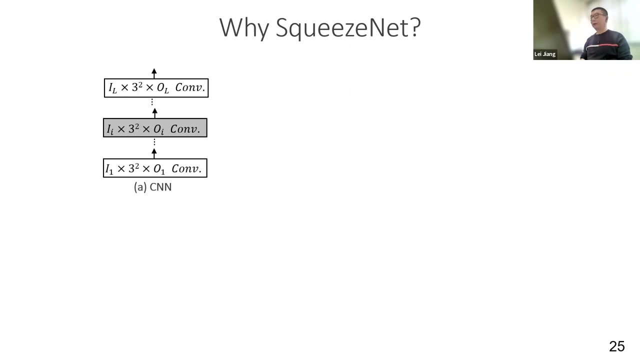 so now the latency gap between the plan test inference and the fhe based inference to around 85 times. so the eva actually take advantage of the mobile neural network architecture to reduce the rotation and the multiplication inside a neural network. particularly, the eva take advantage of so-called a squeeze net to do that, the squeeze net actually. 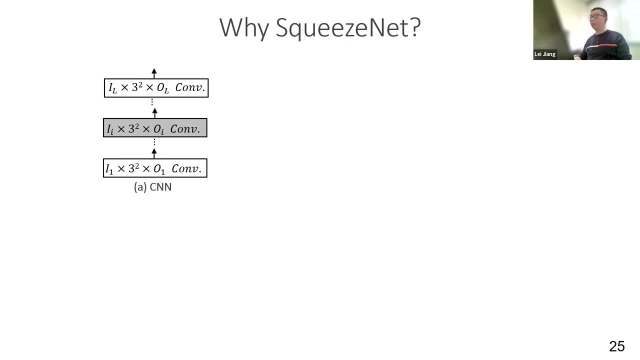 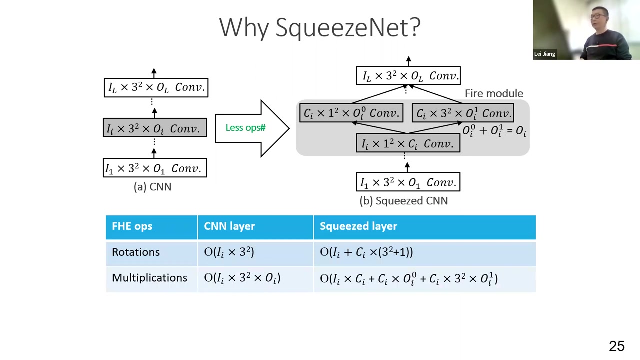 convert a convolutional layer- these are very large convolution kernel- into two different layers. each layer now has a much smaller kernel and maybe much smaller input channel number. so at least the comparison between the a convolutional layer and a squeezed net layer in this table. we can see that by using the mobile neural network. 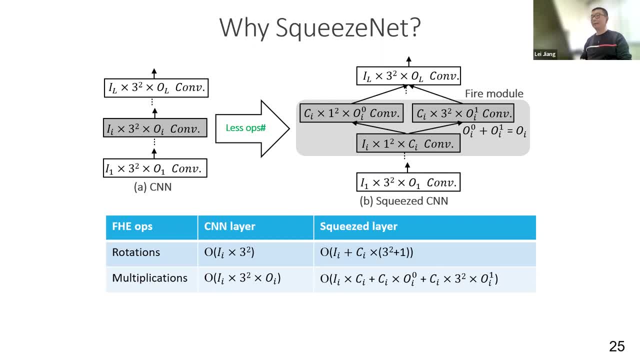 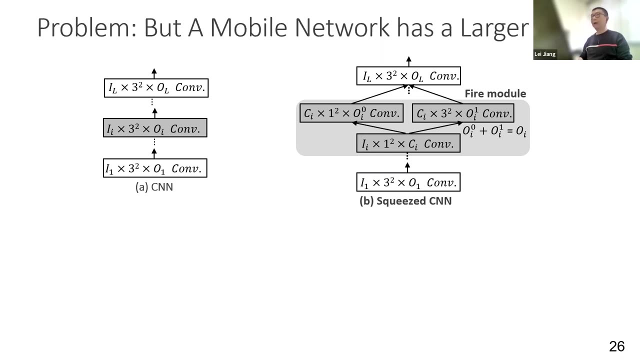 it can significantly reduce the rotation number and the multiplication number in a fhe based neural network. this is the reason why eva can achieve latency reduction. however, eva didn't consider a fact that the fhe is actually very sensitive to its computational depth, so original originally for a convolutional layer. the computational depth of fhe is just one. 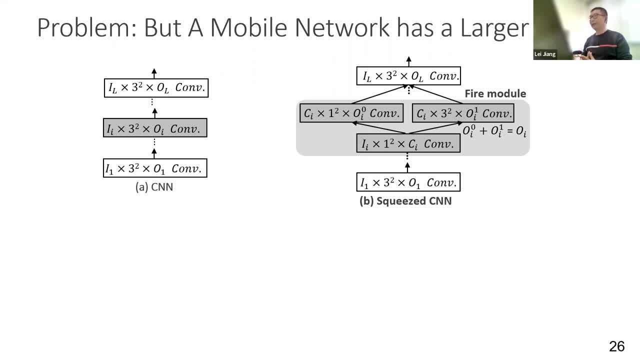 however, if we apply the squeeze net layer into this network architecture, then we actually we actually doubled computational depth. so a double the computational adapts will increase the computing overhead of each operation in a fhe based neural network. here is the computing complexity of a multiplication, addition and the rotation of a fhe based neural network. 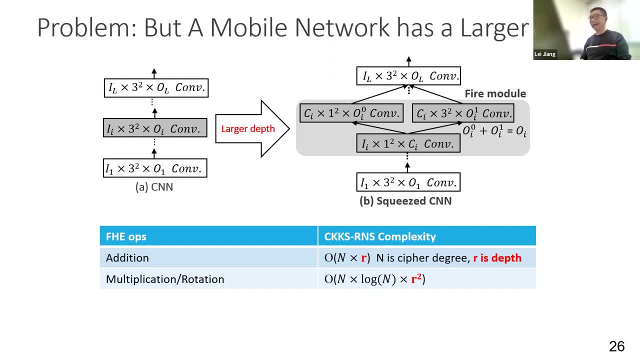 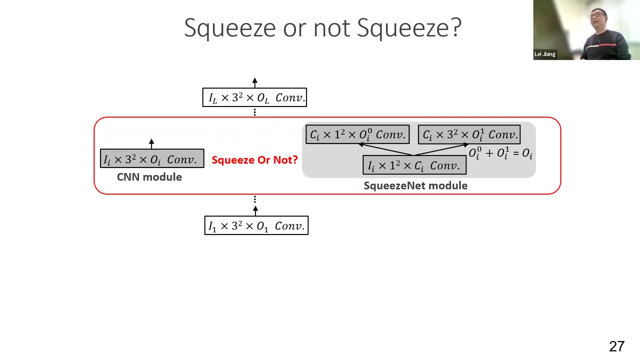 we can see that the complexity of addition is actually linear scales with the computing depth and the complexity of a multiplication and the rotation of FHE is actually linear scales with the depth square. So a larger depth actually makes every FHE operation slower. Then we design the FHE neural network architecture. we will have a problem. 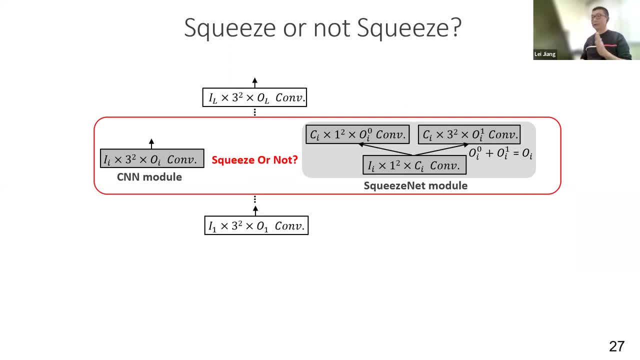 We can choose to use the normal CNN layer or squeeze net architecture. If we choose the CNN layer then we have a smaller computing depths. each operation will be faster. But if we choose the squeeze-net architecture then expectations will change. is not layer. we have a less number of operations inside this layer, but each operation may be slower. 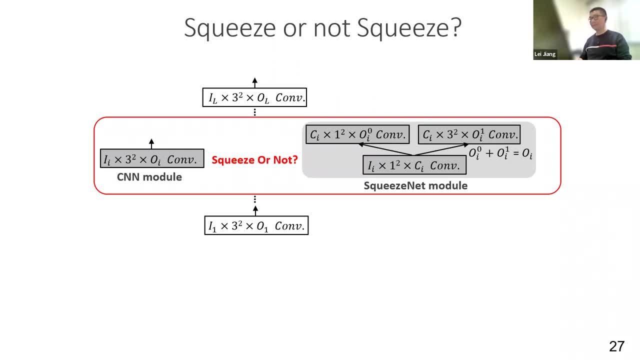 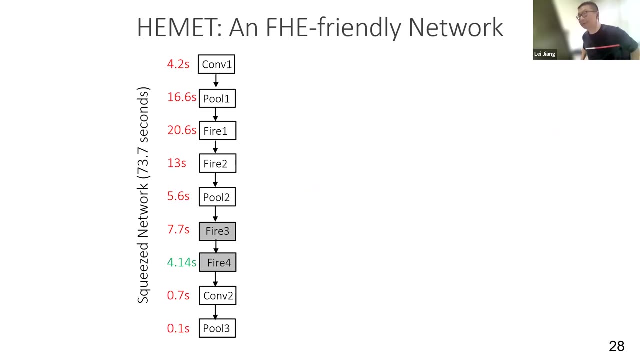 due to the increased computing computational depth. so whether we do the squeeze or not is a problem. uh, for the eva, it accepted the first and the last convolutional layer and i use all squeeze net layer in the middle of this neural network and we run the neural network on our cpu baseline. 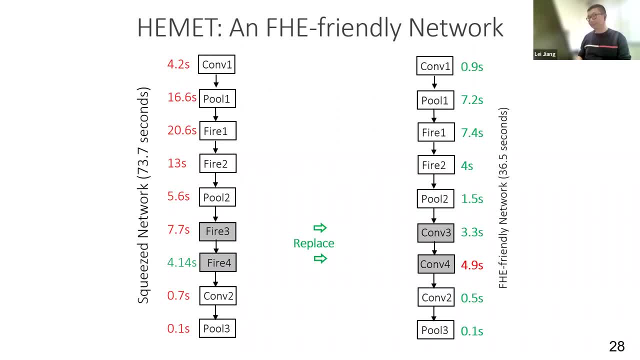 and the record all the latency overhead here. so we didn't propose any fancy search algorithm. we just try to replace the squeeze net layer- here we call it a fire module- by convolutional layer and then check whether we have a latency reduction or not. after we try all the possibilities here, we find out that for the first several layers 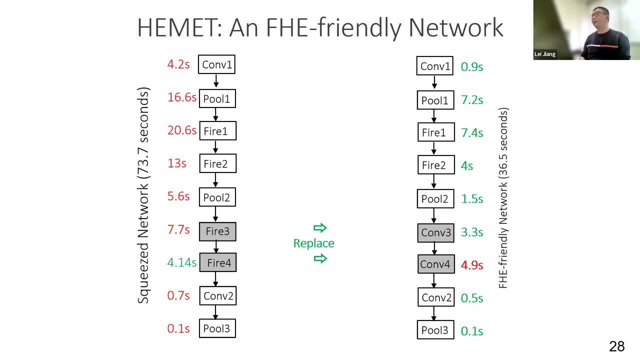 because they have very small computational depths. we definitely prefer squeeze net module or squeeze net layers. however, in the last few layers we should use cns because the double the computational depths will significantly increase the overhead of each fhe operations. here. in this case, we definitely want to have a more operation, but you know each operation should be. 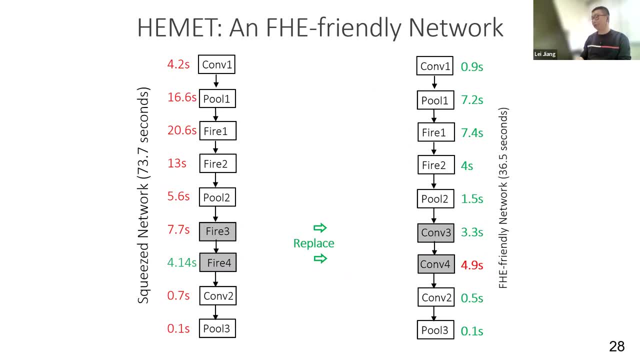 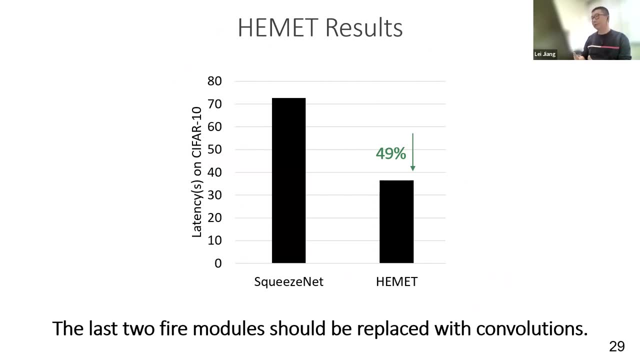 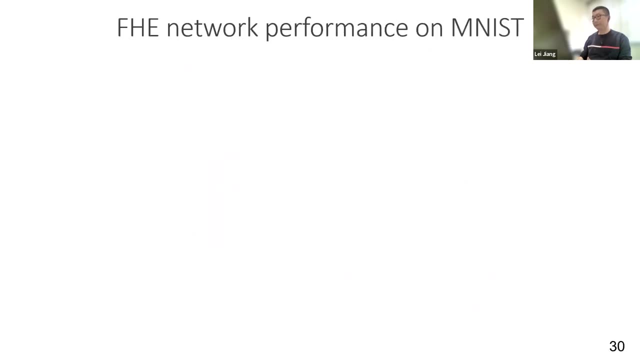 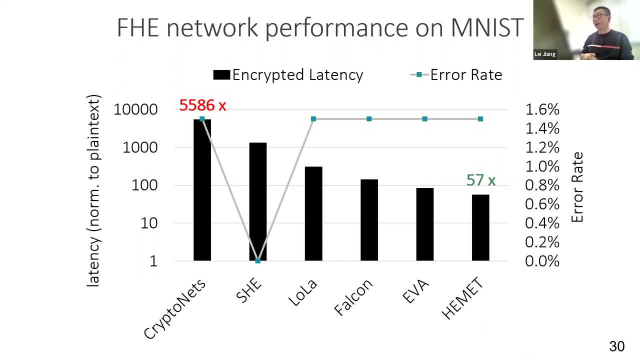 faster. this can be achieved by the convolutional layers. by this thing simple scheme, we can reduce the latency on c4 net image by almost 50 percent. so i summary, so i summarize the result of three of our algorithm level work. in this figure only our first technique. she can actually increase the accuracy of the fhe based on your network. 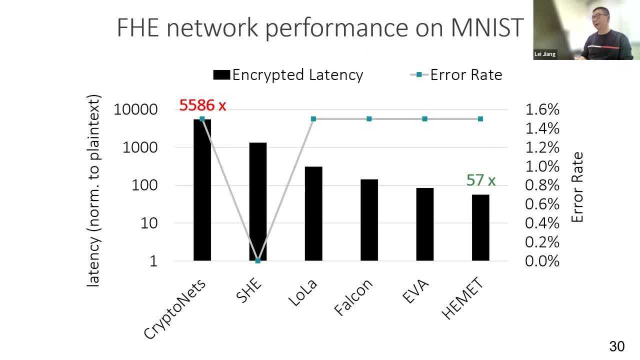 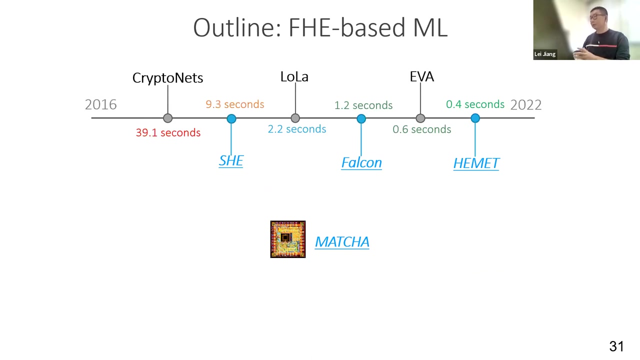 because we do have a more accurate activation operation. for all the other two works, they can only reduce the latency but achieve the same accuracy. now we actually reduce the gap latency gap on the amnesty image to only 40 times. so i have done the three algorithm level work. um, you can see that one inference: 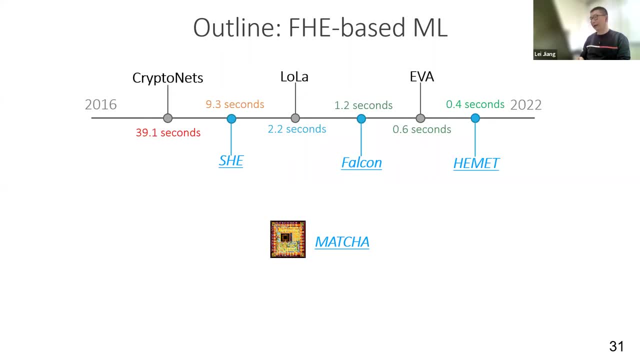 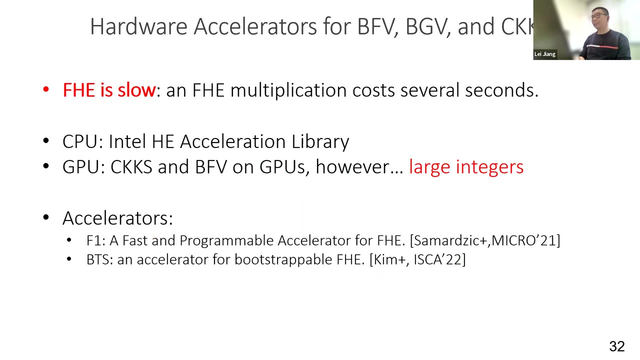 still cost a 0.4 second, which is a very slow actually. that's the reason why we are using this, the reason why we want to propose some hardware specific, some application specific hardware to accelerate the fhe based on your network because of the speed of fhe based scheme. 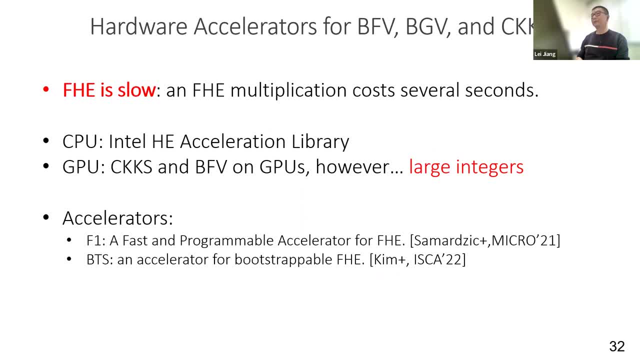 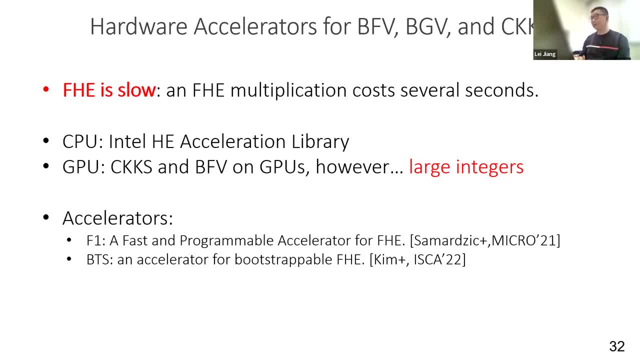 intel created their own libraries so that they can use the long avx-512 instruction to accelerate fhe operations, and people also try to implement a different fhe instruction fhe scheme on gpus. however, the the difficulty here is that gpu cannot support large integers. 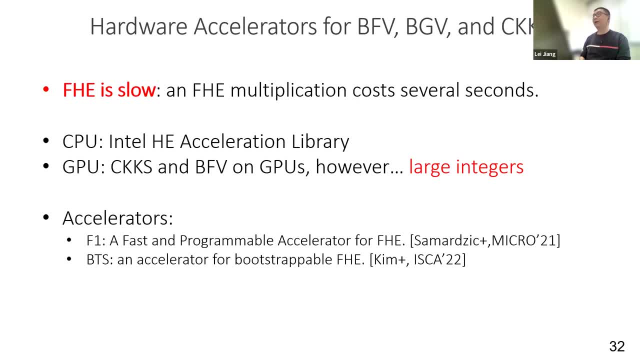 although nowadays gpu can support 8-bit or 16-bit integers, gpu cannot support a 128-bit integer, so it's not very easy to implement fhe on gpus. on the contrary, recent work proposed multiple FPGA-based or asic-based accelerator for fhe based neural network. 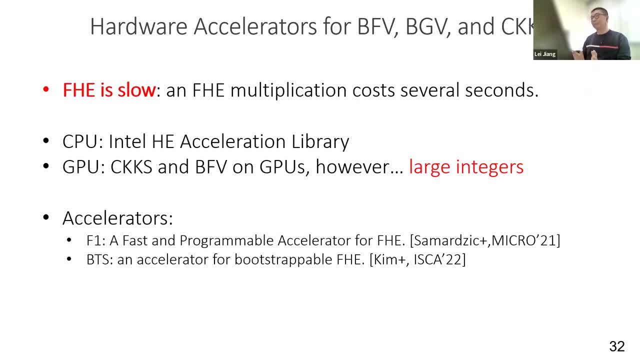 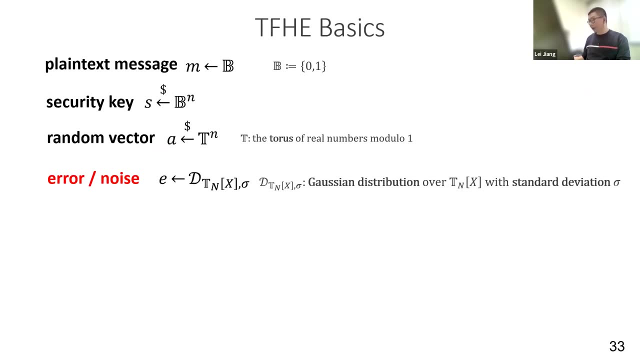 here are two examples, but both of them only accelerate the so-called worldwide fhe based scheme such as bgv, bfb and ckks. so in this talk we propose the first fhe based accelerator features for fhe-based neural network, first accelerator for tfhe, which is actually the bitwise fhe scheme, because it's bitwise scheme. 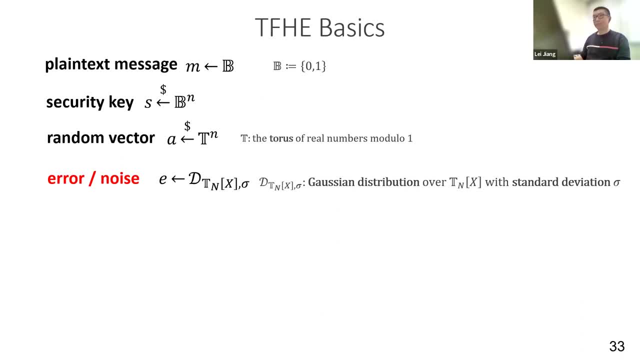 the plant has the message can be only one and zero, and then we need to randomly generate a secret key and a random vector, and these two actually are polynomials- their degree- and we also need to sample some noise during the encryption. we need to add some noise into the plant test message. 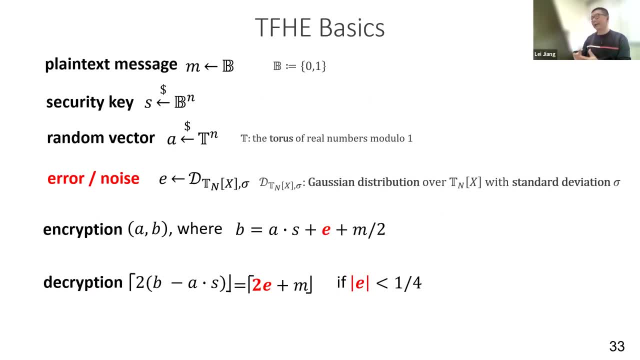 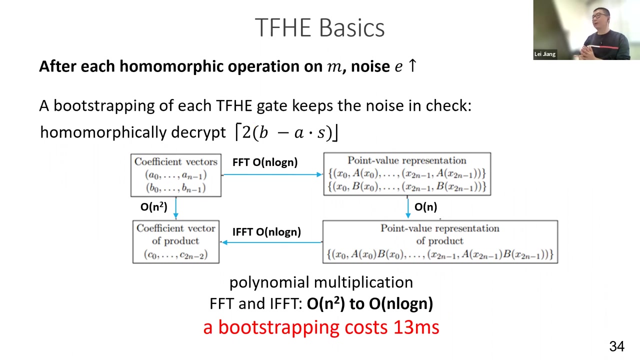 so that we can, you know, actually hide our message, real message, inside this line during decryption. we need to round this noise off to correctly do the decryption. if the noise is very large, we may have a decryption failure in this case. so each homomorphic operation, like a none gate, all gate, will increase the noise a little bit. 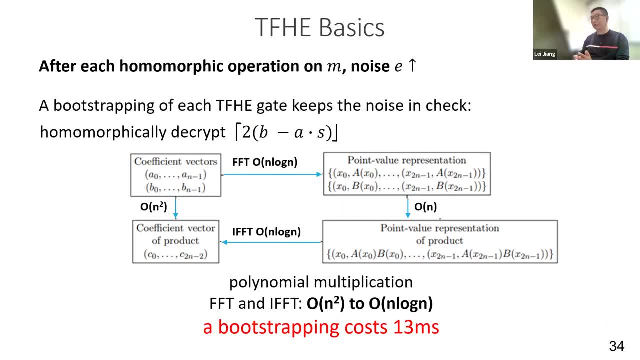 that's the reason why at the end of each logic gates we need a bootstripping to keep the noise in check. you can consider the bootstrapping as homomorphically decrypting this cipher test and remove the e, which is the noise. so the bootstripping involves a lot of polynomial multiplications. 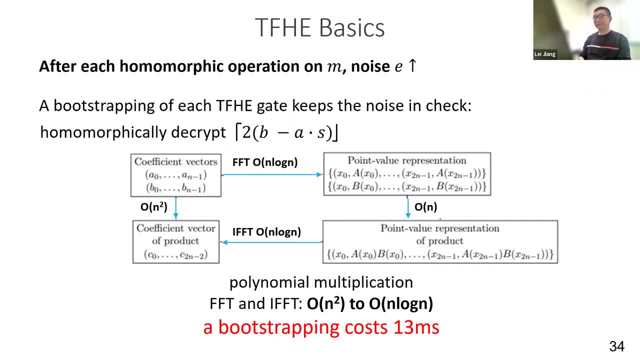 if we directly do a polynomial multiplication, the time complexity is n square r. here n is the degree of the polynomial. however, if we apply fft on each polynomial and then we only need to do coefficient wise multiplication on them, so in this way we can reduce the polynomial multiplication time complexity from n square to n log n. 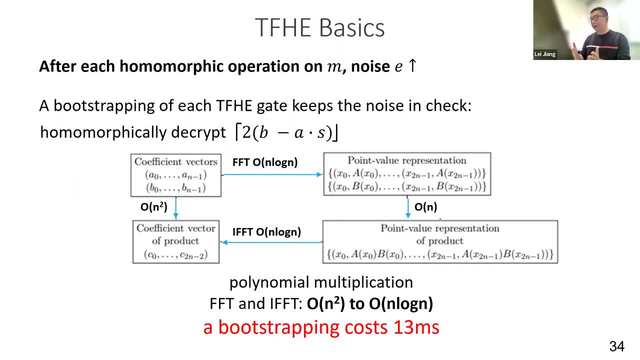 although we have already used fft and irffd, the bootstripping is still very slow. each bootstripping costs a 13 millisecond. you can see that if you have a computer whose gate can, each gate will cost a 13 millisecond, this cpu will be very slow. 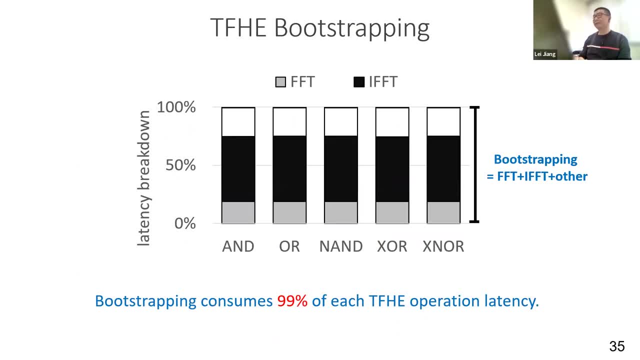 the frequency of the cpu will be very slow and such cpu is even smaller than one megahertz. and then we do some benchmarking on the different tfg logic gates. we find out actually the bootstripping operation dominates the gates. it costs 99 percent of the latency in each operation, particularly fft and irffd. 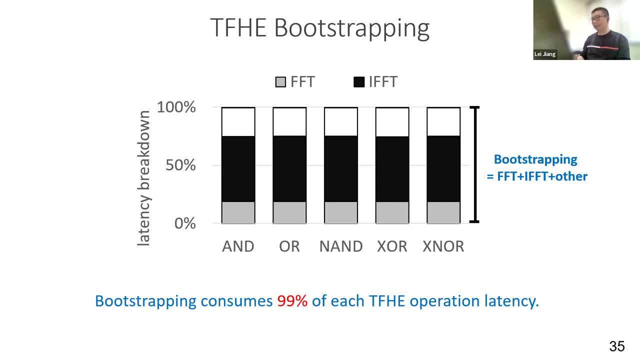 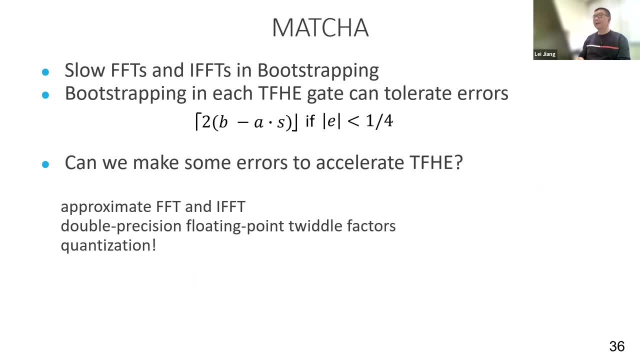 are very tight consuming in the bootstripping, So the FFT and the IIFT are very slow in the bootstripping and the bootstripping can help the gate and, to you know, tolerate some errors. Inside each gate we have a bootstripping and this bootstripping can reduce the 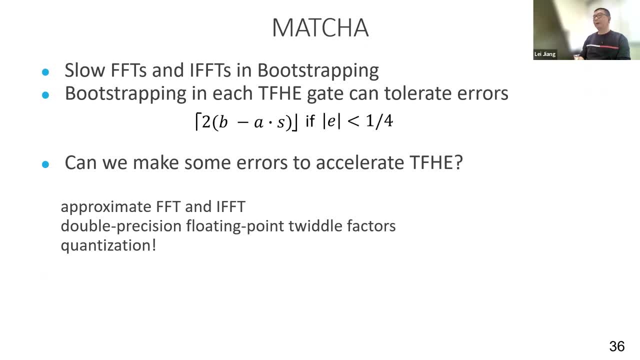 errors, Which means that can we actually intentionally generate some errors to accelerate the bootstripping? The answer is yes. We can try to use approximate FFT and inverse FFT to accelerate the bootstripping. We need to make sure the error does not, you know. 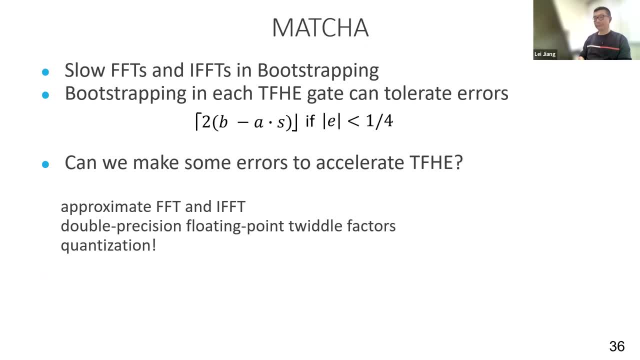 be larger than some threshold. if the error is smaller than some some threshold, we can do some composition on the total factor of the FFT and the IIFT. So in this way we can reduce the power consumption of each FFT and the IIFT unit in the in the accelerator and try to have 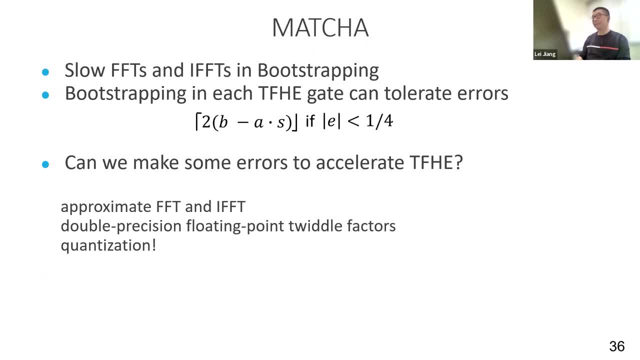 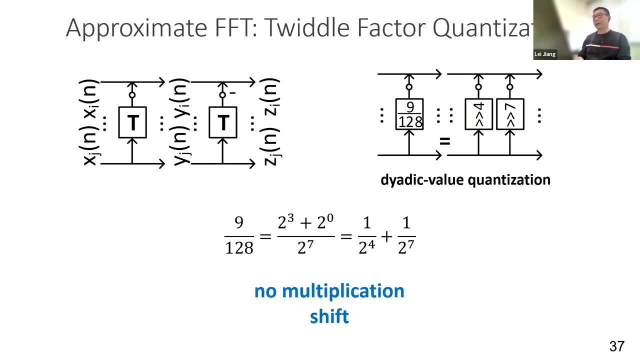 more computing units with the same power budget. So here is the flow of data, flow of the FFT. in a bootstripping We can countize the total factor into some that dyadic values. For one dyadic value each number here can be break into. 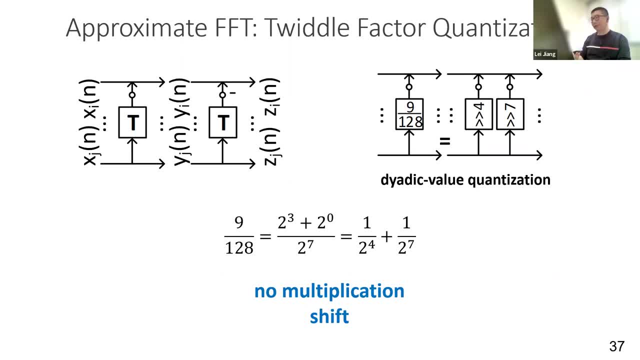 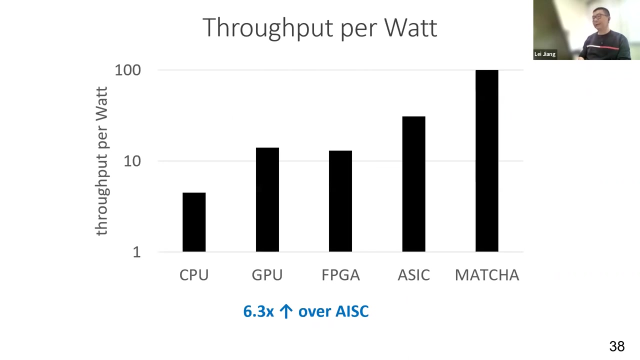 the combination of some two to n representations. When the number can be represented by two to n representations during the multiplication we only need to do the shifting, binary shift. This is similar to our first technique, SHE. By the simple quantization on the total factor we can. 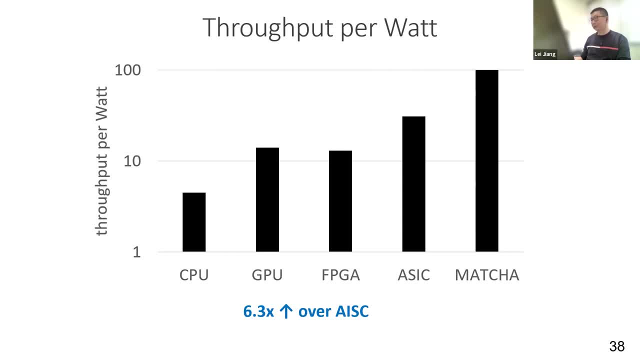 significantly increase the bootstripping throughput Compared to the latest FFT. we can increase the bootstripping throughput By the simple quantization on the total factor. we can significantly increase the bootstripping throughput By the simple quantization on the total factor. we can significantly increase the bootstripping throughput. 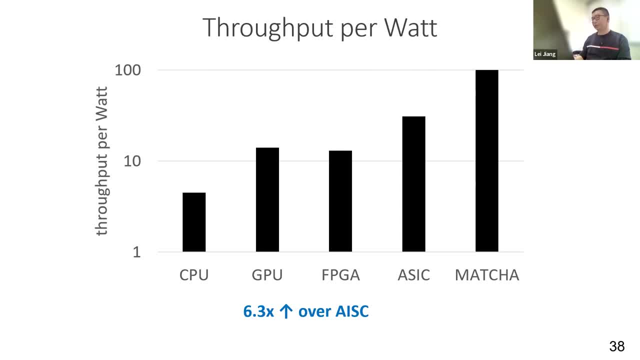 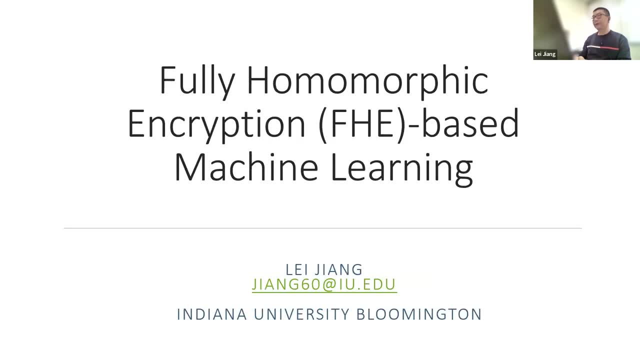 The latest ASIC accelerator we can increase the throughput per watt by more than three times. So in this talk I introduce three algorithm level work to increase the accuracy and reduce the latency of fully homomorphic encryption based neural networks. We also propose a accelerator to accelerate. 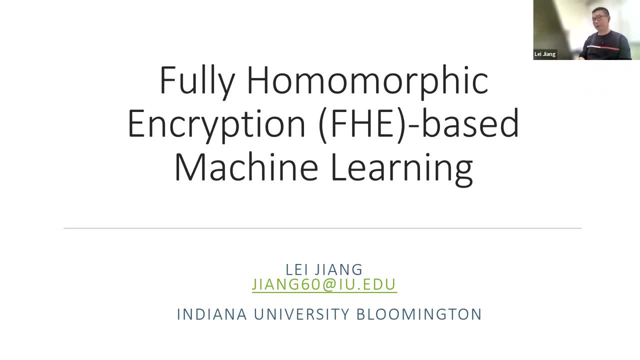 We also propose a accelerator to accelerate than your network. Thank you very much. Thank you, Lei. Thank you very much for a wonderful work, And actually I have several questions to ask, but before that, so I would like to offer opportunity to our audience. 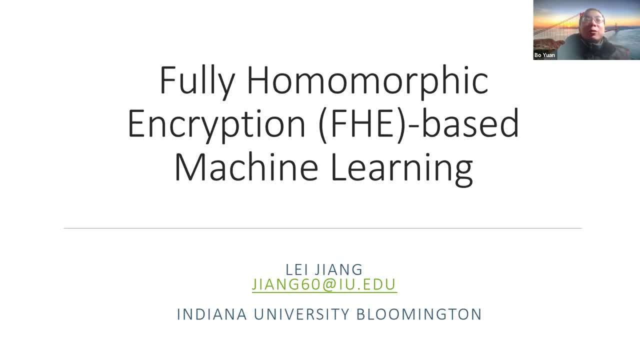 So any questions from our audience, So you can unmute yourself or input a question in the chat box. I think I can, maybe I can. Yeah, I think- I have one question. Thanks a lot, Professor Jiang, and thanks a lot for the nice presentation. 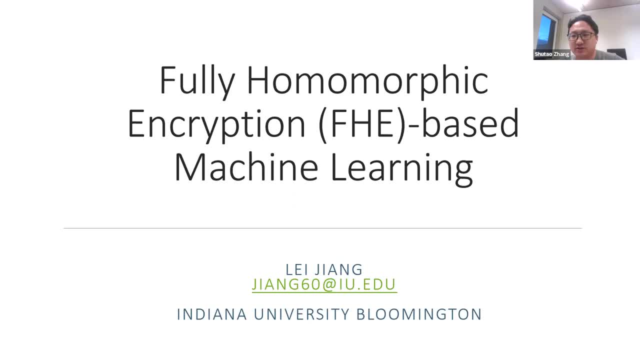 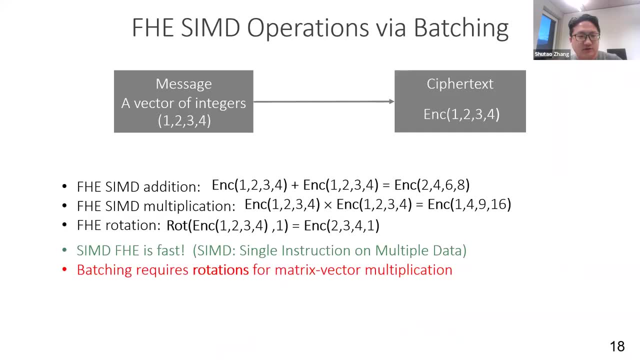 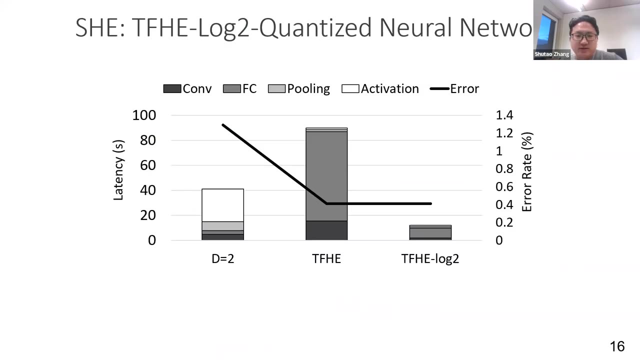 I have one question regarding the page 16, regarding the first work, the quantization, oh sorry, the activation function is accurate for this scheme. I mean, I don't even know why. Can you please explain this? Can you repeat the question again? 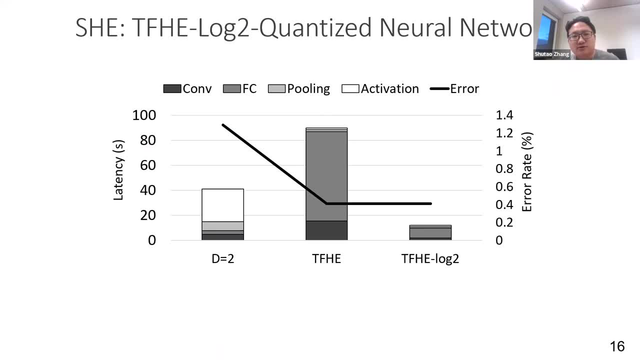 In this SHU scheme the activation function, a homomorphic encryption scheme- is accurate for high final accuracy. So I didn't realize the reason for this. Can you please explain? Can you please explain this So by the? this is very good question actually. So by using the binary homomorphic logic gates we can implement a accurate ReLU operation. So these ReLU operation are very critical to the accuracy of the neural network. Although we do some log2 quantization in the convolutional layer, we can still achieve the same accuracy. 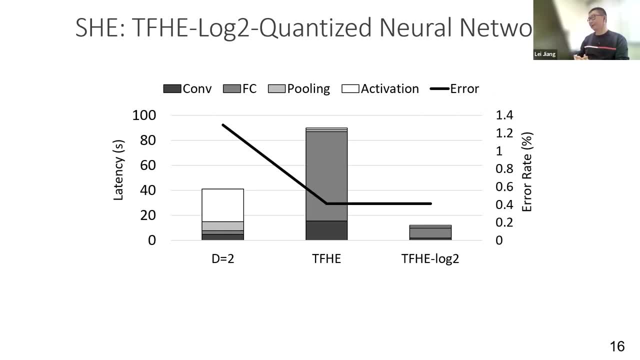 as the original TF-HE based neural network. Did I answer your question? Maybe one more question regarding this. In the plain text domain example we have that ReLU, just a two piecewise linear function. right, But is there some special representation? 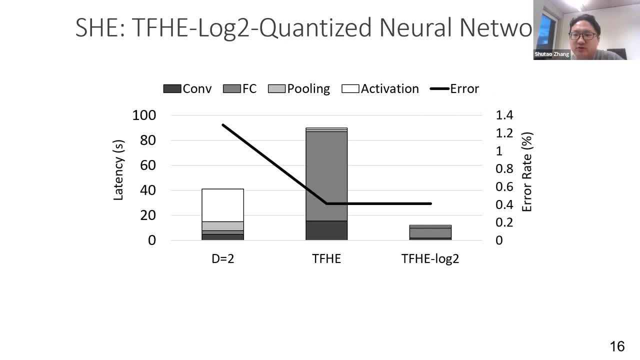 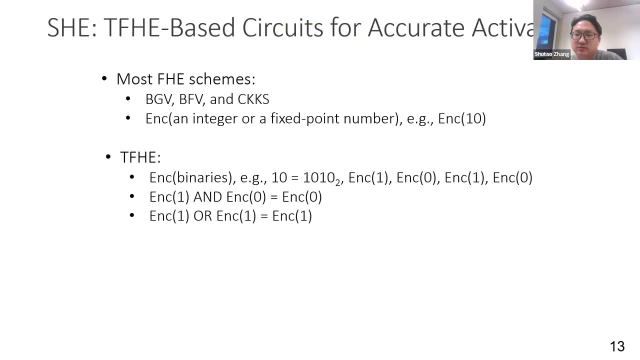 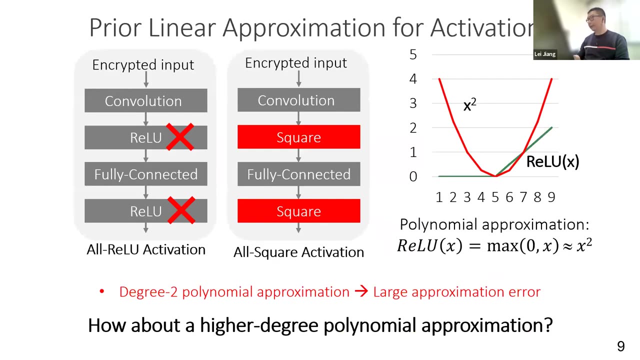 in the cipher text domain. for this, The ReLU is a non-linear operation. okay, Yes, yes, Although you can use a polynomial to approximate the ReLU like this: In this example, they use a square degree two polynomial to approximate this ReLU. 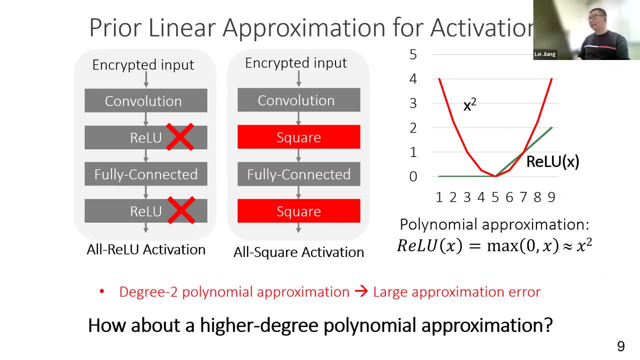 Yeah, yeah, Yeah, yeah, You can now have this ReLU. They have some differences. You can try to increase the degree, approximation degree. You can use x2, five, x2, 10, you can do that, But again the approximation result is not good. 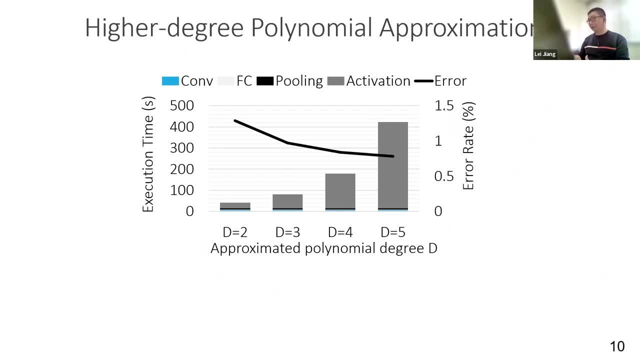 be tried the degree five, although the error rate slightly goes down. This is good. this is an advantage. All right, um, the latency significantly increases if you use fhe to compute a such high degree. uh, polynomial, the overhead is very large. okay, thanks a lot for the explanation. uh, maybe one more question. uh, this slide is pretty nice. 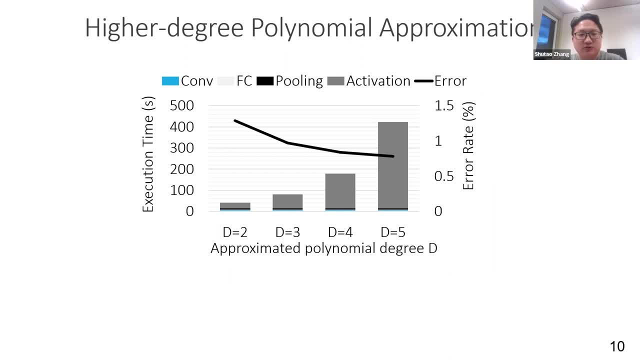 and including much information meaningful to, i guess, to us. oh so, can we get access to these slides somewhere? no problem, no problem, yeah, so so the uh, so the entire talk will be recorded and uploaded to the youtube. yeah, oh, youtube, okay. okay, that's pretty nice, thank you. 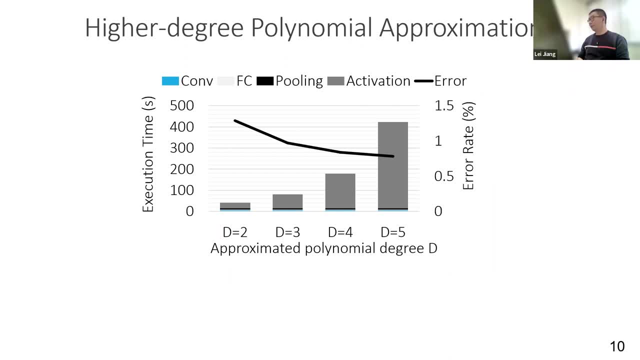 thank you a lot. thank you, other questions from our audience. so actually i have some questions, yeah. so first a very wonderful talk and i was. i was wondering so whether if we use some other type of activation function instead of a loop and then we can like to achieve kind of good balance between the latency and the accuracy. 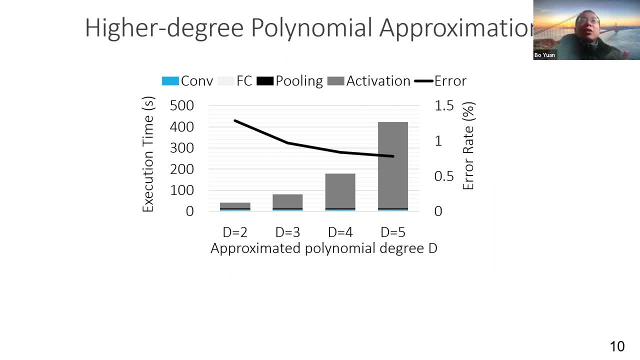 right now, for example, as these slides show that, so very initial effort that we want to use some the higher degree of polynomial approximation to approximate the reform. but if we like to replace a room for some, use some other, like the leaky rule or some other activations. 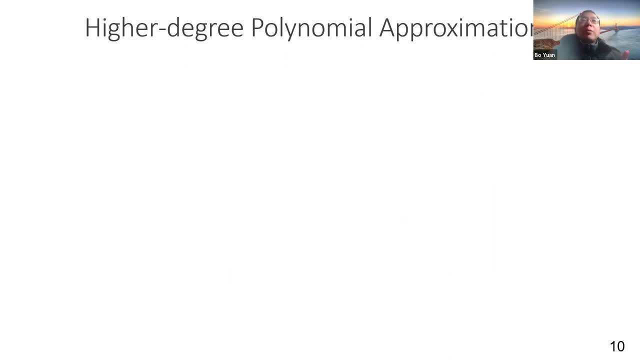 whether the performance we can achieve, kind of better balance or trade, okay, anything else, not for this book. this piece points: uh yeah, some other things that i think that we can use for some take back. finally, thank you. uh yeah, plentyضi, i did uh nito today. if you could just give my hand card. uh, this was also for those of you that like find a student, tell you more details about elements etc. stuff for derivatives, if you kind of like. 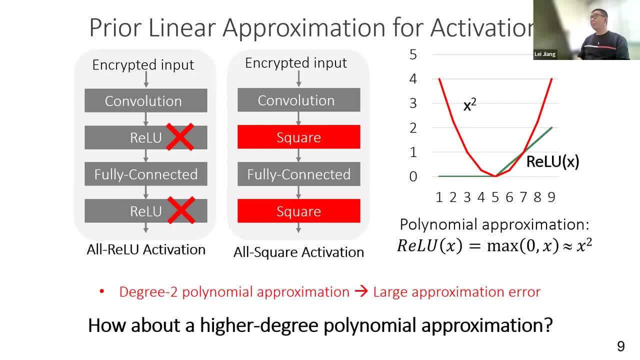 This is a very good question. actually, ReLU is the simplest activation for modern neural network. Of course we can have more advanced activations, but all the activations here are non-linear operations. So, for example, you mentioned the Leaky ReLU, Leaky ReLU actually. 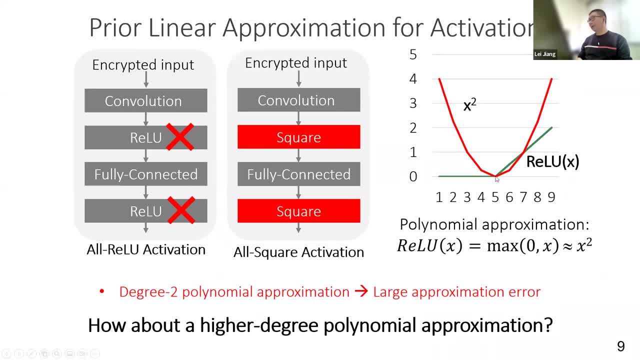 needed to compare multiple points Here. we only needed to compare against zero. If it's larger than zero, it acts itself. Otherwise it's zero. So the comparison inside FHE is actually very difficult. That's the reason why and people. 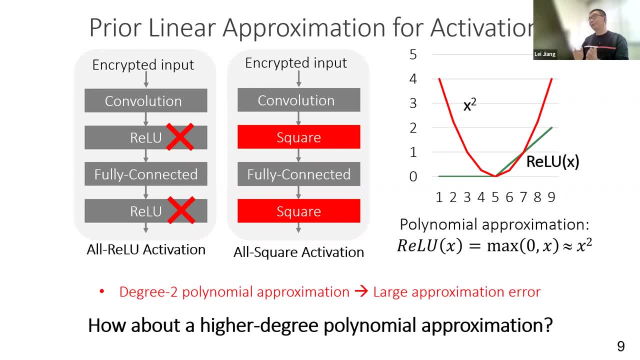 try to use square to approximate that For the Leaky ReLU. we can definitely use TFHE to implement that activation, but we need to use more comparison operation to achieve that. It's slower but I think you can have a very good accuracy improvement. 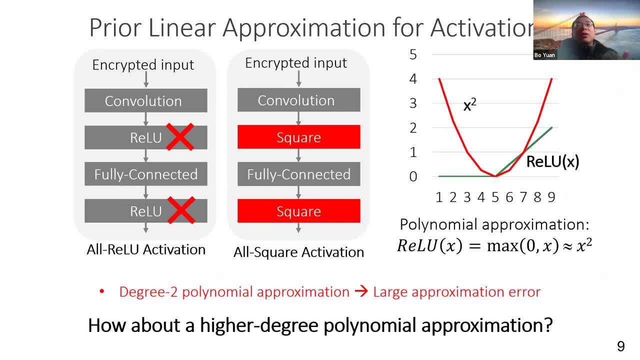 And another question is that right now it looks like in the algorithm community, right now all the experiments are based on an M-list and so on. so how about if we further scale up the dataset? So, for example, right now it is doable to 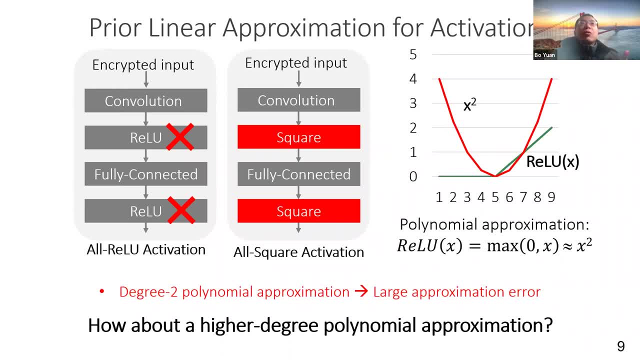 do experiment for the FHE-based neural network, like CIFAR-10 and even for the ImageNet. But if it has come too slowly or Yeah, The speed is not the first concern but the nonlinear operation on large-scale neural network. 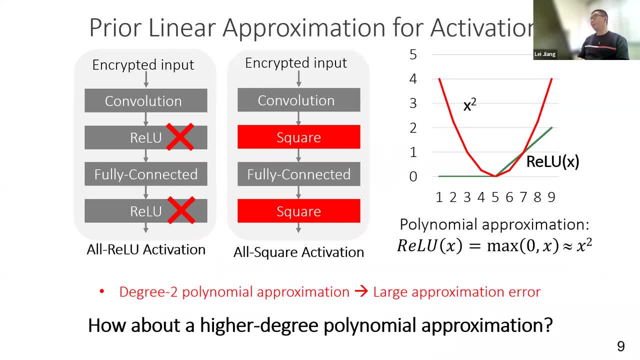 is the biggest issue. If you do not have nonlinear operation for ImageNet-scale neural network, the accuracy is not very good. But now the FHE can handle CIFAR 10 or CIFAR-100 level dataset already, But for ImageNet it's very challenging. 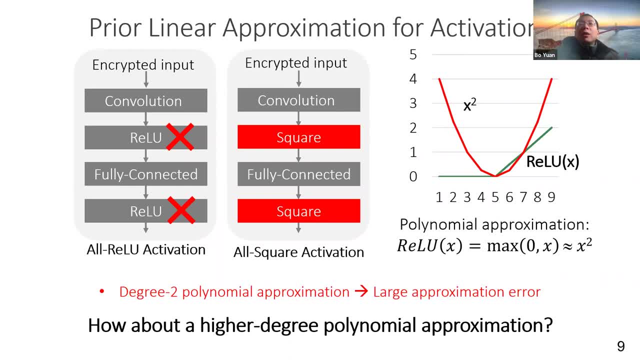 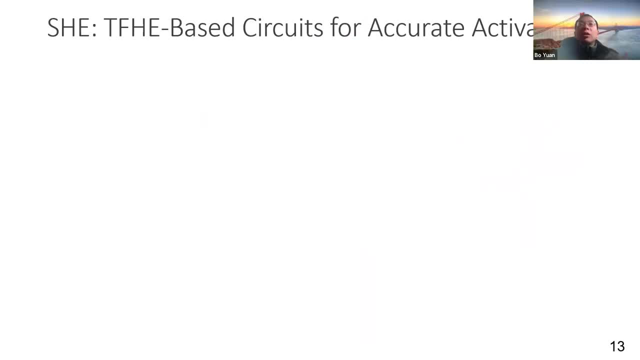 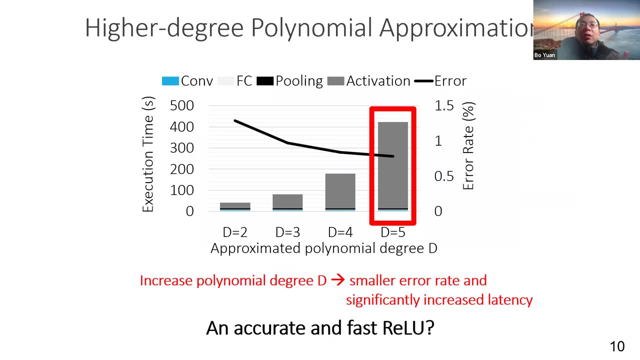 Another question is that: so I remember that you have one table. Yes, You have one table that shows that for the speed on the plain text. so for the MNIST it's a very, very fast one, Right? Yes, yes, yes. 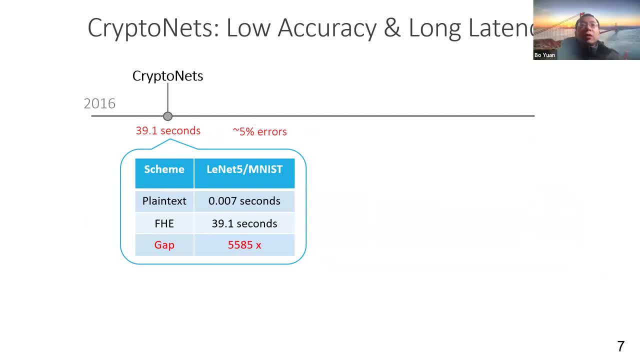 It's the latency actually. yes, Yeah, yeah, 0.007 second, And for FHE it's about 40 seconds, And so, based on your optimization and so on, so right now we can reduce to like the second level. 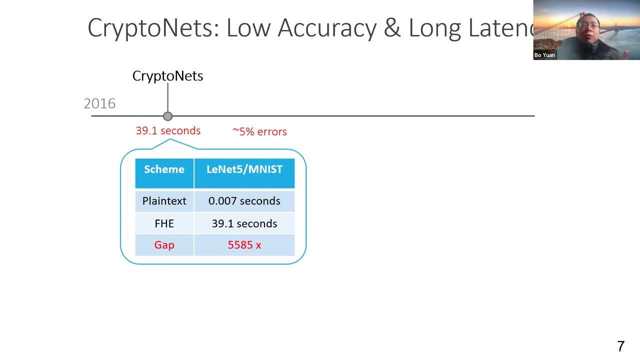 So I was wondering, so, whether we can obtain the further improvement via like. So whether we can obtain the further improvement via like to providing more customized the GPU kernel to accelerate the entire inference and so on. Yes, of course, In addition to the algorithm-level optimizations. 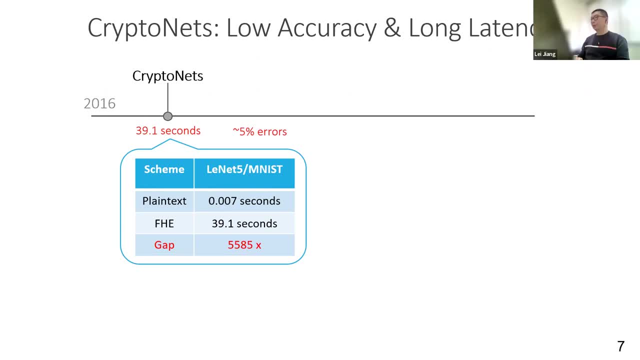 Yes, of course. I believe the reason why now people pay more attention to FHE is that there are a lot of algorithm-level innovations to FHE. is that there are a lot of algorithm-level innovations to FHE? is that there are a lot of algorithm-level innovations? 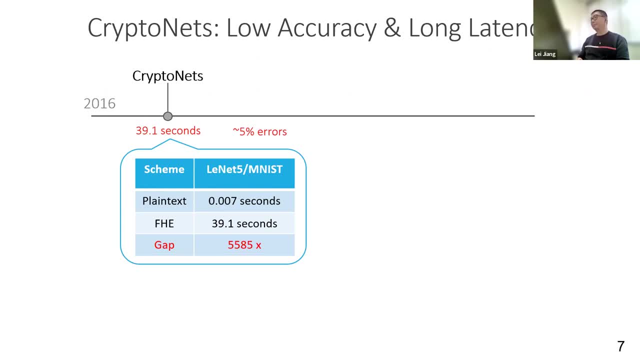 I mean cryptographic innovations. People create a lot of new FHE scheme which are faster but maintain the same security level, And then we have a lot of algorithm level, neural network level improvement And then we can use more advanced architecture hardware. 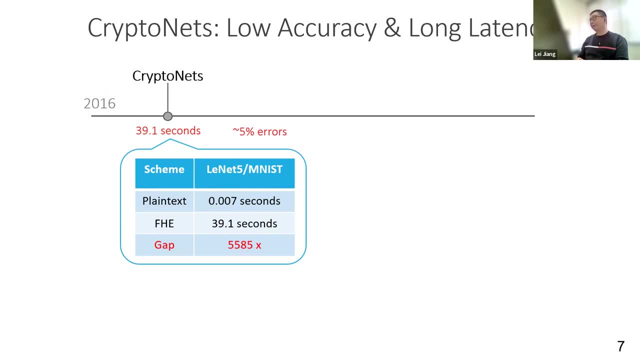 to do the acceleration Now I believe there are a lot of group are working on how to run FHE on GPUs. But again, FHE are mainly about a polynomial, multiplication additions. Those polynomial has very large coefficient. Each coefficient of the polynomial may be 128 bit. 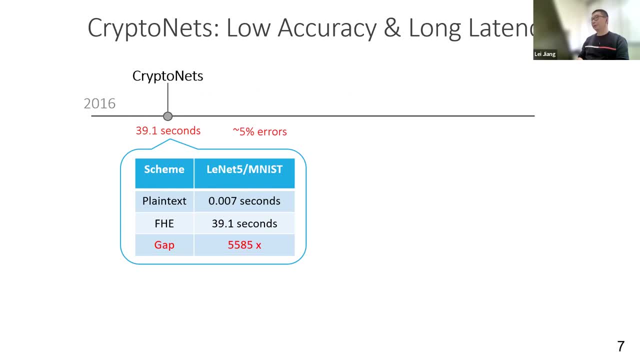 And by the GPU, can now, to you know, support such a large integer well, So that's the reason why more people pay more attention on the FPGA. Yeah, yeah, I know that, like DARPA, they have a, I think about two years ago. 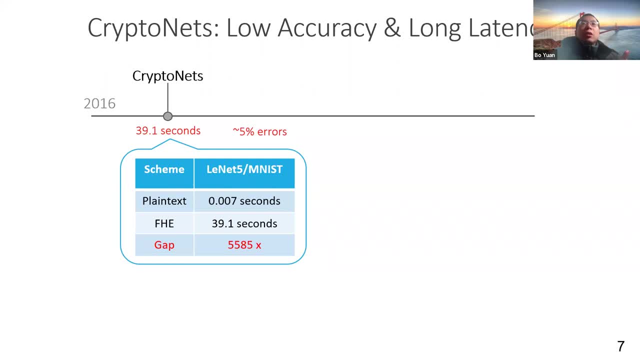 they have a new project to ask the academia and the industry to build some of the ASIC chip to accelerate the FHE right. I remember that Even there's some stuff in the Silicon Valley also working on that. Yes, yes, I have some additional questions. 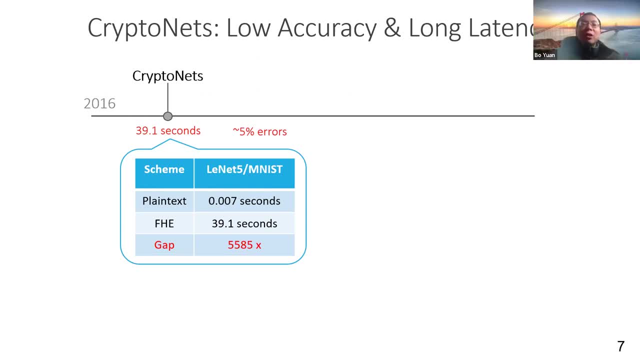 but first, is there any other questions from our audience? Oh, I have a following question regarding to the large data set. So you're talking about so for now, the FHE can now deal with the large data set like the ImageNet. 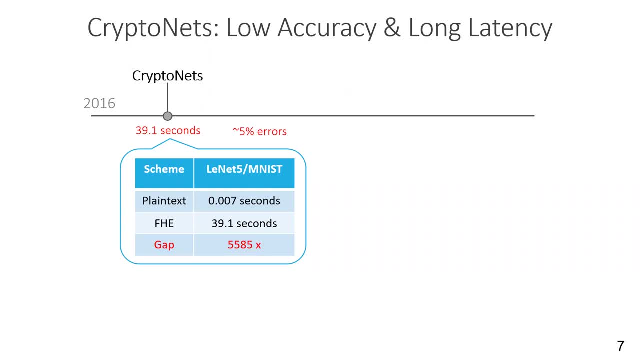 So when you talk about it, I'm wondering: you mean that the accuracy will be lower or the latency is very, very large? Yes, yes, The latency is compared to the plan test. of course the latency is very high. 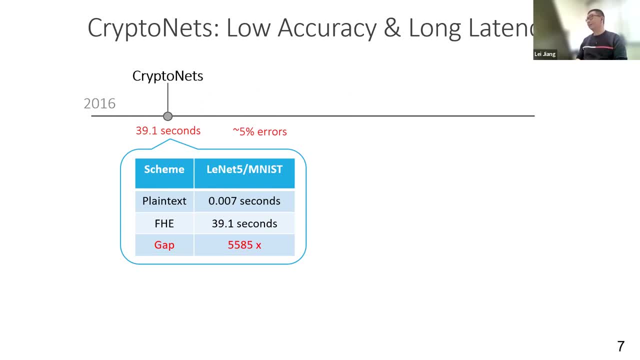 This is for sure, But the long latency is still tolerable. The downside, the major difficulty, is the accuracy. because you don't have, you know, accurate, nonlinear operation. It's really difficult for FHE to support ImageNet at a scale network. 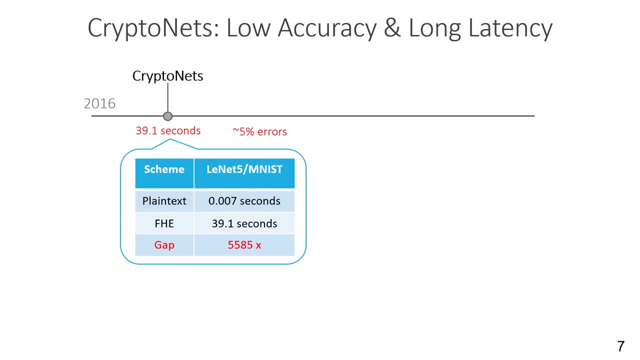 OK, so my understanding is that the low accuracy, because we know that for the classification test, the ImageNet classification is more challenging. But when you were talking about the large data set I was thinking about- maybe it's about the data set scale. 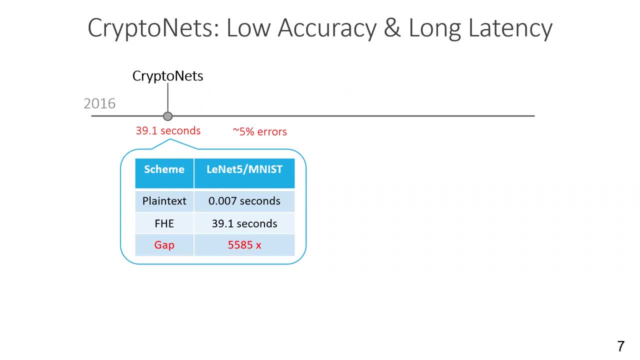 like how many data sets, how many training data sets we have for this task. But for now, from my understanding, it's not. it's not about like there are so many training data sets where the ImageNet input size is bigger than Zephyr 10. 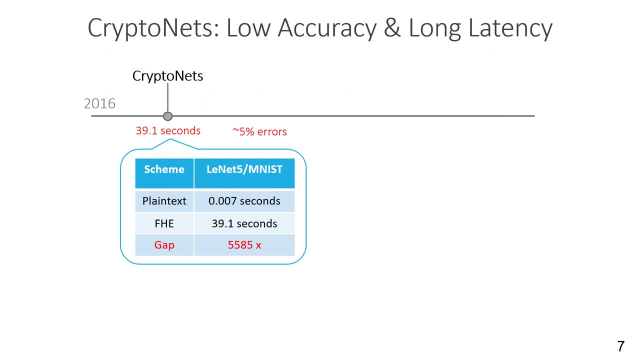 or MNIST. It's mainly about the classification difficulty, right. So it will introduce, though it will cause lower accuracy. That's why we can now deal with it right now. I mean for the FHE, That's right. 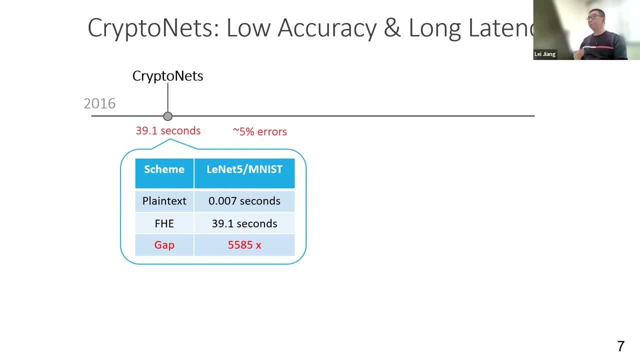 Do I understand it right? That's right, That's right. So, OK, got it, Thanks. Thanks. So for the training data set, it's one issue. After you have your training data set, we can use the accuracy trained by this training data. 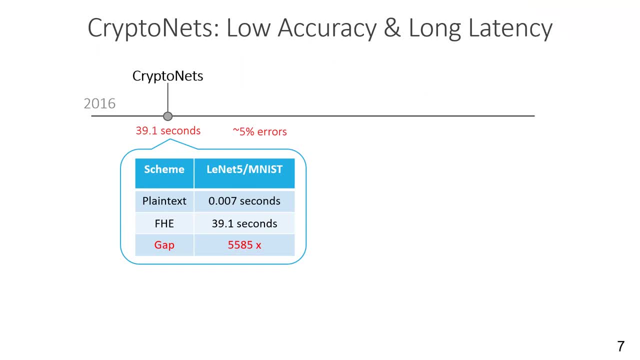 set as one baseline And when I talk about FHE cannot achieve high accuracy. I mean based on this baseline accuracy. the FHE actually will degrade your accuracy because of the lake of nonlinear operations. Yeah, I understand. I get you. 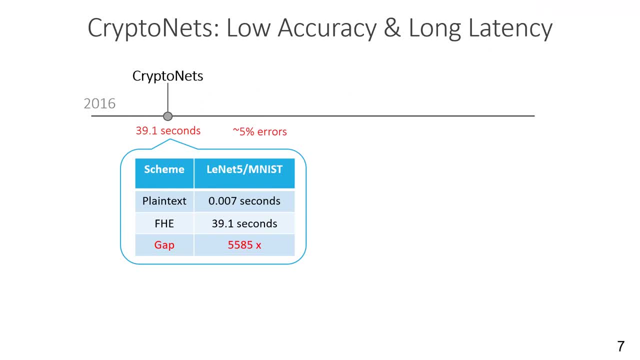 I got it. I can try to figure out the accuracy of the training data sets, But really you can actually experience the accuracy of your training data set levels just by taking the data set and then actually using linear expressions. Oh, OK, OK, I got it. 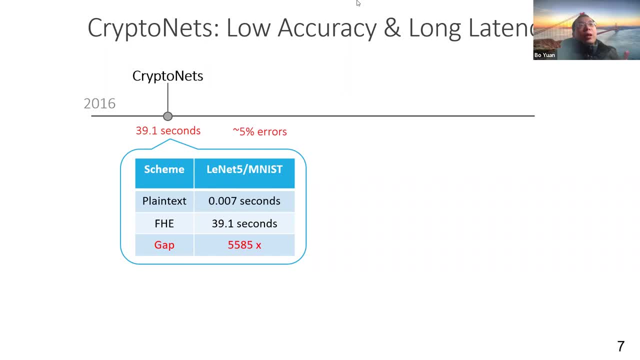 Thanks. Thank you. Other questions from the audience. non-linear activation function for the fhe on the largest scale data set. so i'm just roughly thinking so whether we can just learn the activation function using an additional small neural network to do that and this monitor work. actually it is the relu. we use the relu for that. 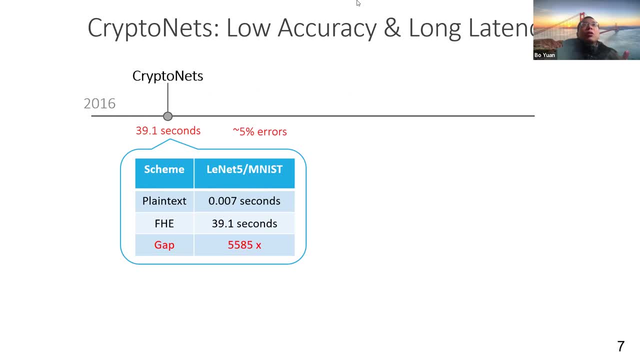 but this smaller neural work actually essentially it performed to just to learn for the non-linearity, for the fhe. so this is just some of some of my very rough thoughts. no, no, this is a very good idea actually. um, you can definitely to fine-tune your neural network. 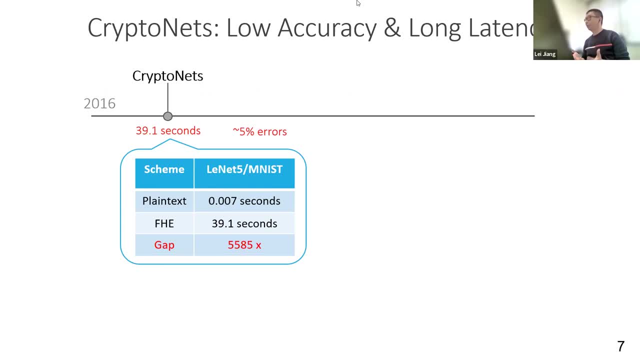 to make the neural network more comfortable. you know, when working with fhe for sure, because you know fhe will intentionally have some, you know- errors. and then your neural network itself can also tolerate some errors, and the error, the error generated by the activation, of course it. 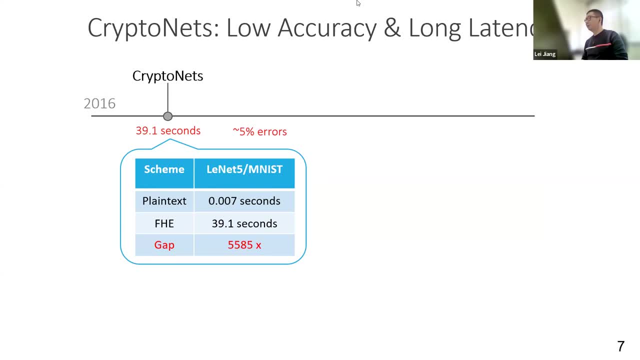 you know can be tolerable by the neural network, no matter you have a smaller neural network for the activation, or, you know, you combine the large and small together. okay, okay, thank you. and the another question is about the use of one slides you mentioned. use the, the circulants, a block circular and the metrics. 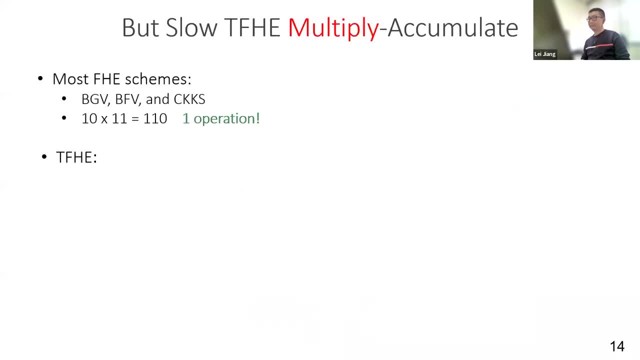 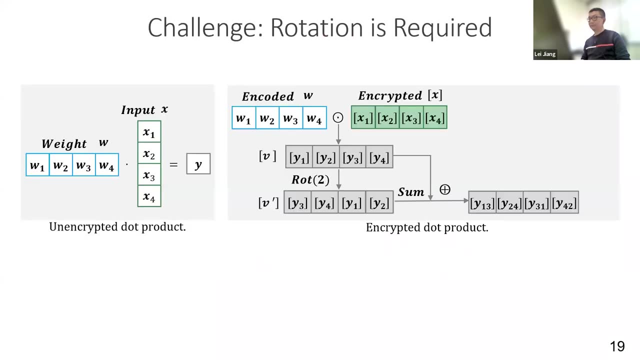 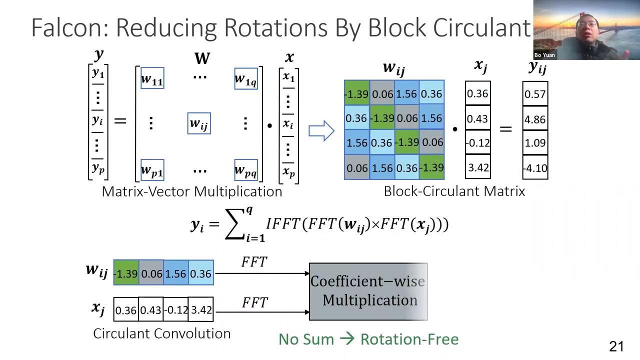 yes and yeah. so here, so for the uh, uh for the block circle, and so i assume that so actually you change the weight of the neural work right to make it to enforce that the block circular and the structure there, right and uh. so my question is that because the the uh for the block circle and the matrix, so the 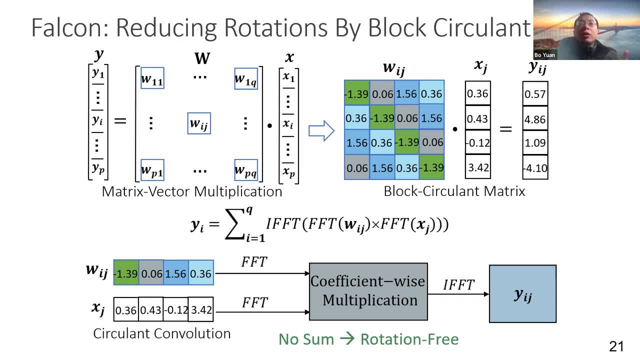 the matrix uh. the fft size is equivalent to uh is equivalent to the block size. so here, so, for example: so so what is the block size do you use here? because we know that when the fft size is, the number of the point of the fft is kind of small. 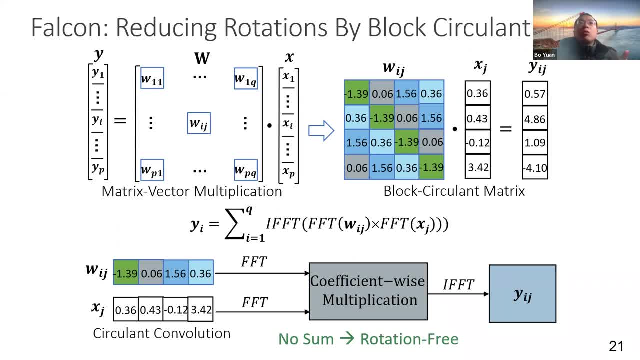 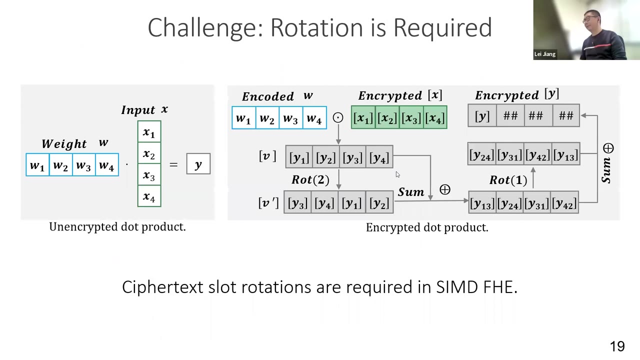 so actually we cannot obtain the considerable acceleration on the gpu or the cpu here. um, the main, the major goal of adopting this block circular and the composition is that we want to reduce the rotation inside each cipher test, and the rotation operation actually is very slow. um, why do we, why do we need a rotation? we, we have to accumulate all the results.